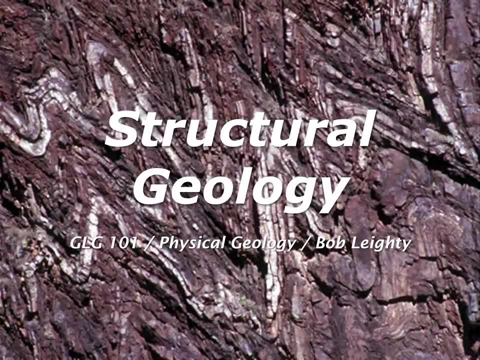 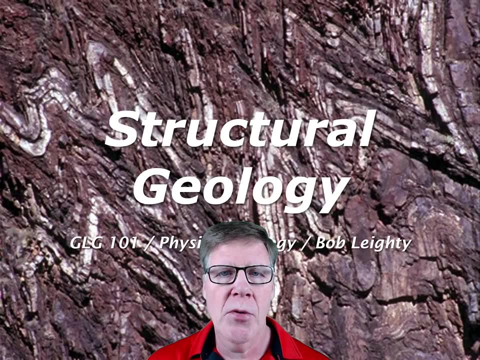 Structural geology focuses on the various types of geologic structures and the interpretation of their origin. Different plate tectonic settings include stresses that may produce a range of these structures that can be generally described as either brittle faults or ductile folds. 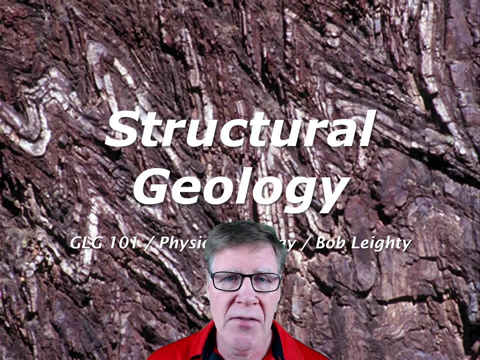 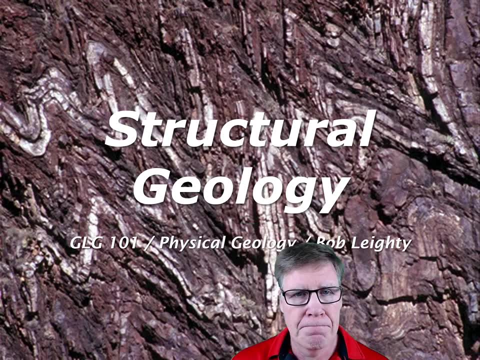 We will review the principal types of stress, tension, compression and shear, and the various types of geologic structures that occur as a result. This is a view of the spectacular fold exposures developed in the Paleoproterozoic Maverick Formation in Barnhart Canyon located. 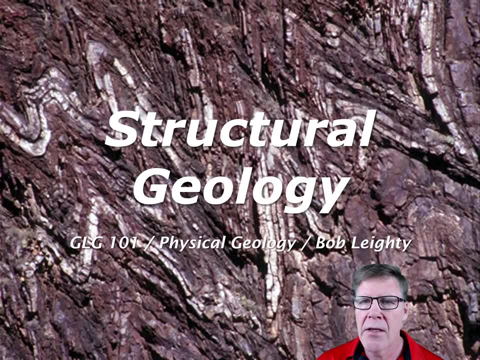 in the Mazatzal Mountains of central Arizona. Here the white, tightly folded quartzite layers contrast with the reddish-brown quartzite and form what are called chevron folds. The deformation that formed these folds occurred during the Mazatzal Orogeny over a billion years ago. 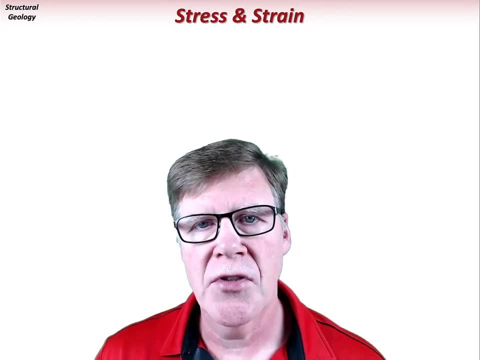 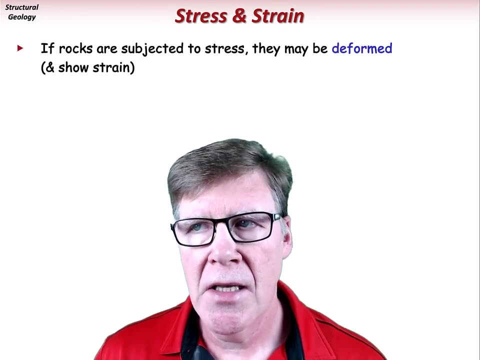 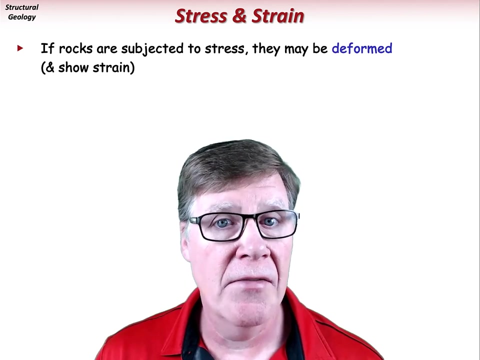 Understanding stress and strain is central to describing and interpreting geologic structures. Simply put, if rocks are subjected to stress, they may be deformed and thus show strain. Stress and strain cause and effect. For example, these flat-lying sedimentary rocks at the top of the 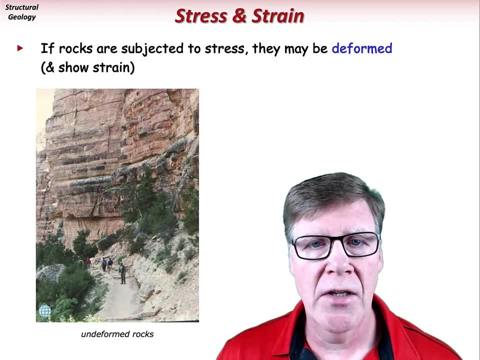 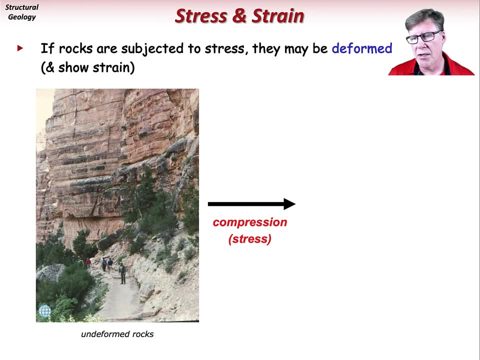 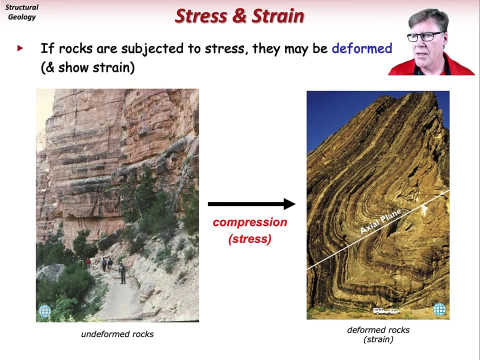 South Kaibab Trail in the Grand Canyon are relatively undeformed or unstrained. However, if they are subjected to compressional tectonic stress over time, they may be deformed and show strain. These formerly flat-lying sedimentary rocks in Namibia have been deformed. 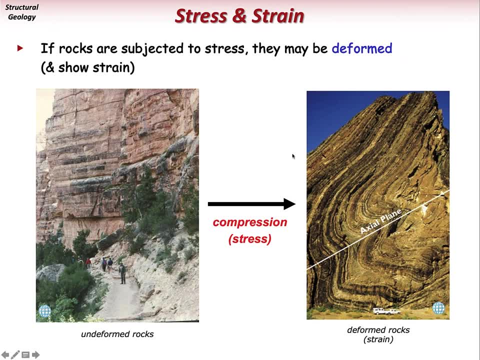 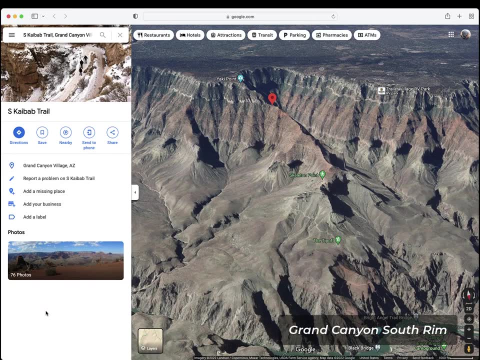 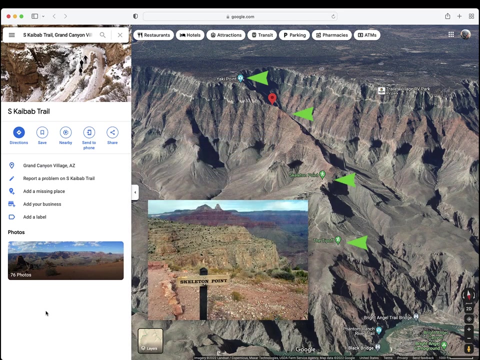 causing them to turn into an overturned fold In the Grand Canyon. the South Kaibab Trail descends through the so-called layer cake formed by the more or less horizontally oriented Paleozoic strata and starts at Yaqui Point, progresses down through Cedar Ridge, Skeleton Point and the tip-off on its way to the inner. 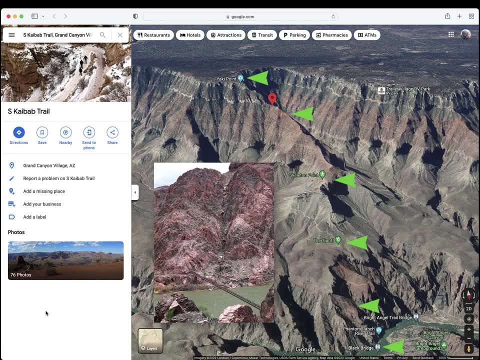 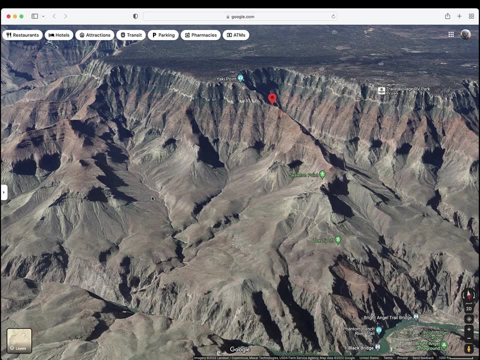 gorge, where it then crosses the Colorado River at the Black Bridge on its way to Phantom Ridge. The South Rim of the Grand Canyon is underlain by the Permian-Kaibab Formation and in this area forms the edge of the Coconino Plateau, which is part of the much larger Colorado Plateau. 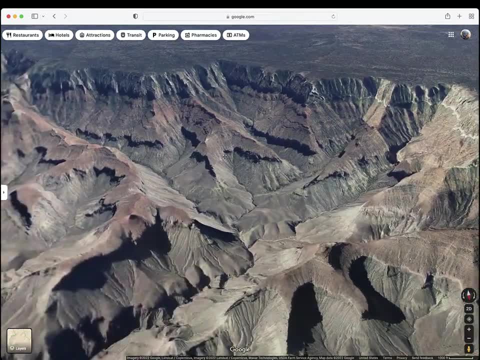 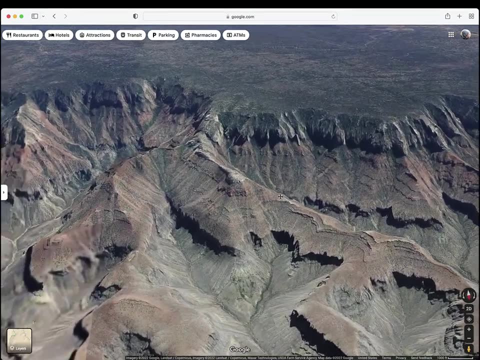 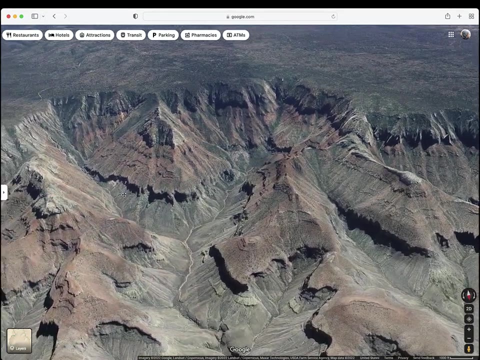 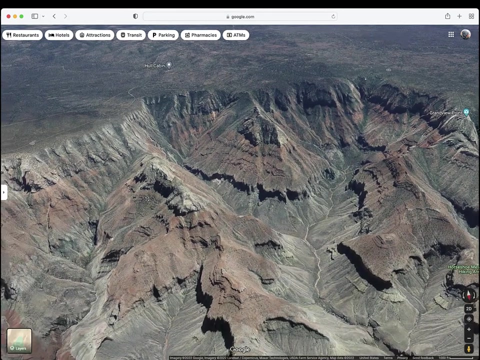 Across the Colorado Plateau, including places like the Grand Canyon. the geology is largely characterized by relatively flat-lying Paleozoic and Mesozoic sedimentary units that have not been significantly deformed since their formation millions of years ago. Only locally have these strata been deformed into folds called monoclines. 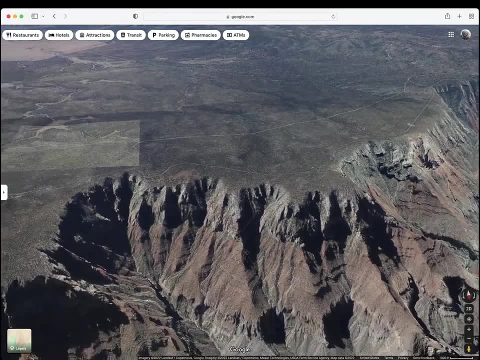 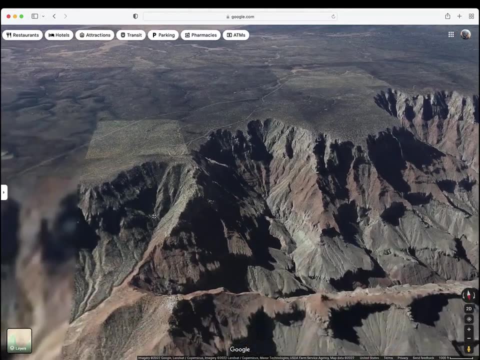 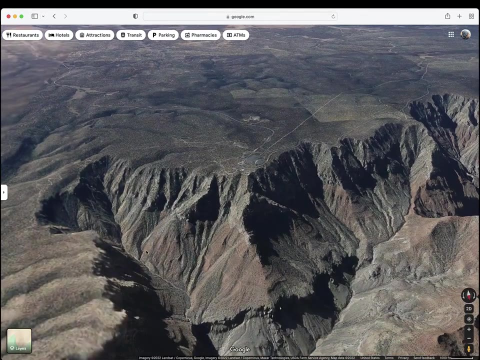 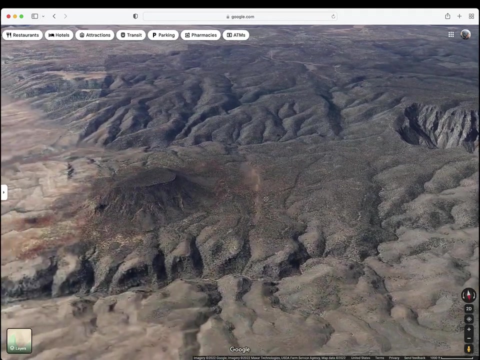 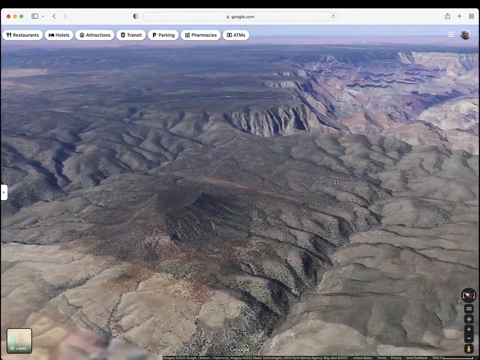 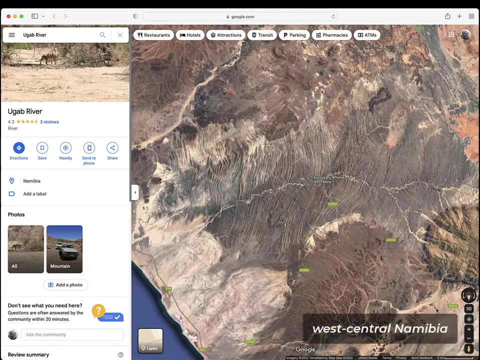 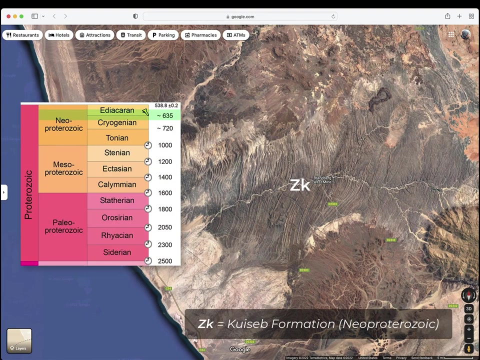 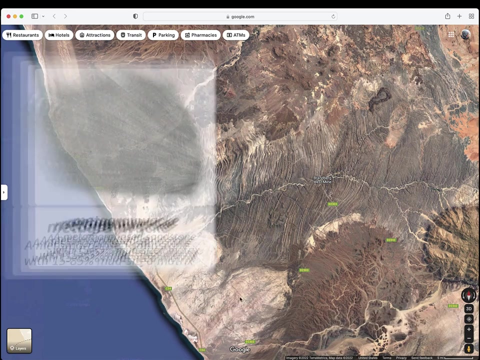 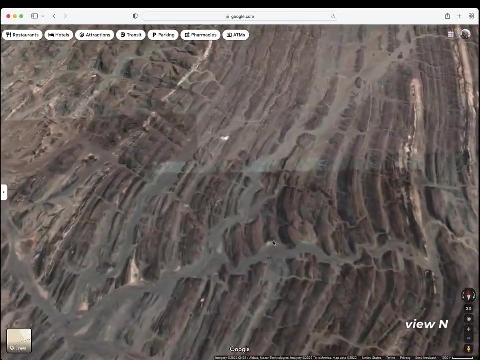 This layer cake stratigraphy and the high desert climate produce spectacular landscapes, plateaus, mesas and buttes. The this area here is the lower Ugob River area of West Central Namibia, and here the late Protozoic Kuiseb Formation represents a considerable thickness of folded metamorphic greywacking. 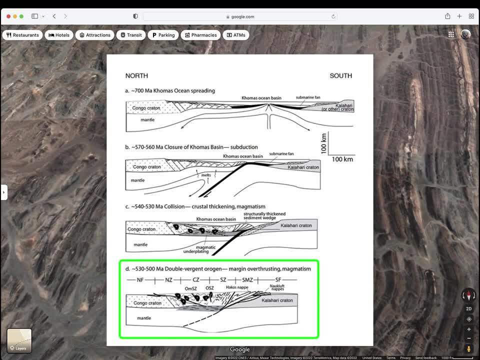 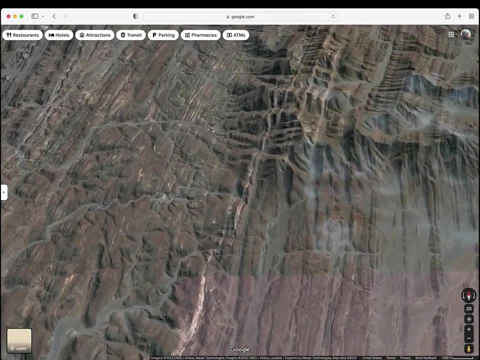 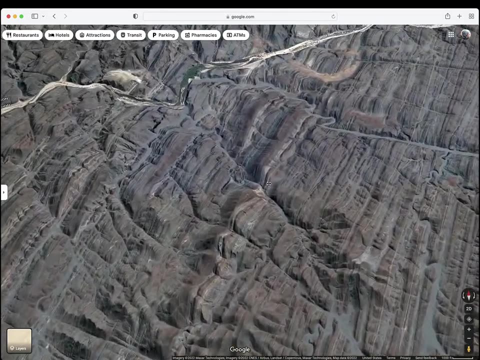 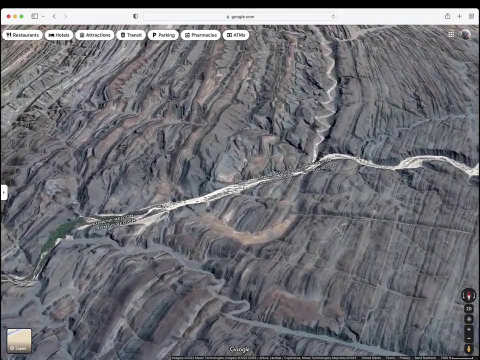 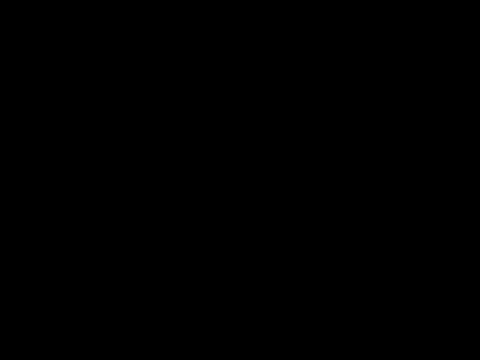 system that was deformed during the Cambrian collision of the Congo and Kalahari cratons. The region displays evidence of four phases of structural deformation, from open folds to tight to isoclinal folds. There are three basic types of tectonic stress: tension, compression and shear. 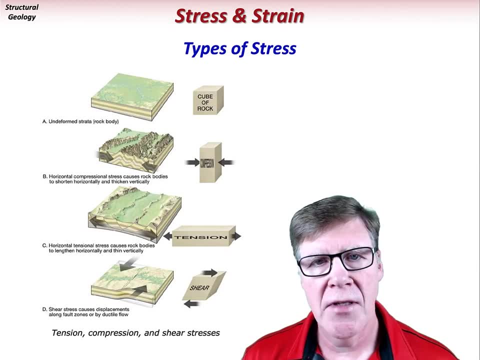 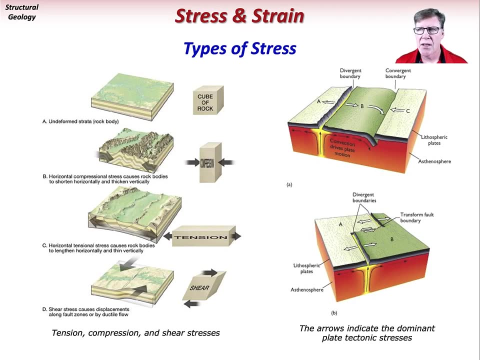 This diagram shows the three basic stresses and their effects on geologic layering. This diagram shows the basic tectonic settings where these stresses dominantly occur. The first situation shows horizontal layering, where the rocks have not experienced any tectonic stress. 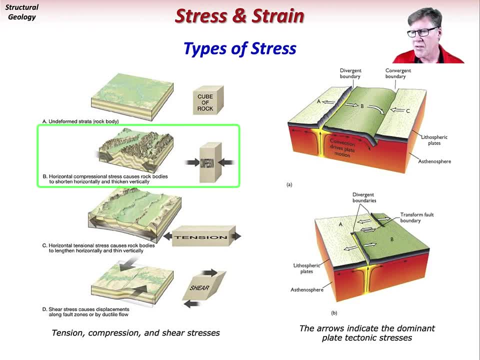 and thus no signs of strain. In the next example, compressional stress includes opposing forces that cause rocks to shorten horizontally and thicken vertically. This is the dominant stress at convergent plate boundaries, where tectonic plates are moving toward each other, And you can see that on the right. 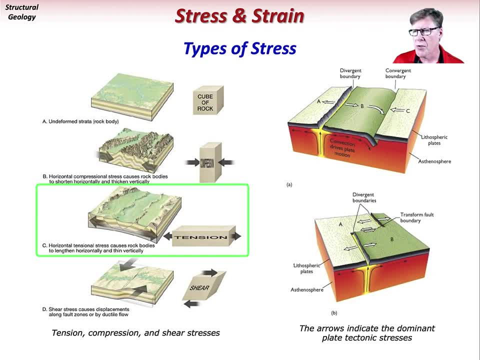 Tensional stress includes opposing forces that cause rocks to lengthen horizontally and thin vertically. This is the dominant stress at divergent plate boundaries where tectonic plates are moving away from each other. You can also see that in both diagrams on the right. 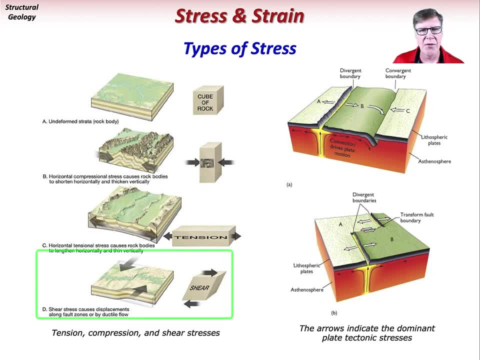 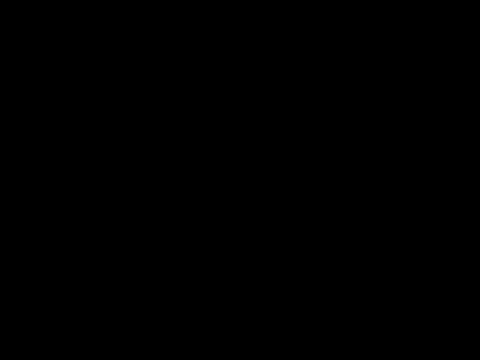 Sheer stress includes opposing forces moving in opposite directions. This is the dominant stress at transformed boundaries where tectonic plates are moving side by side past each other, And you can see that in the bottom diagram on the left. There are two stress sources at convergent plate boundaries that cause rock to tighten horizontally. 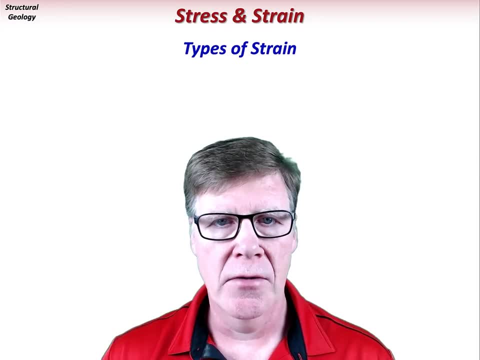 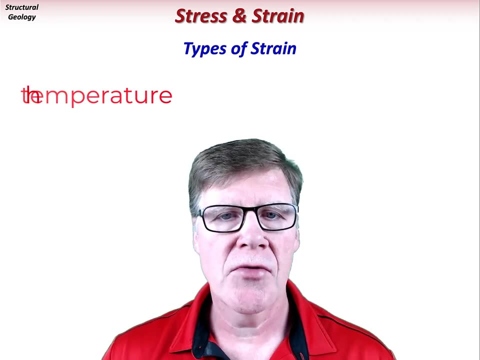 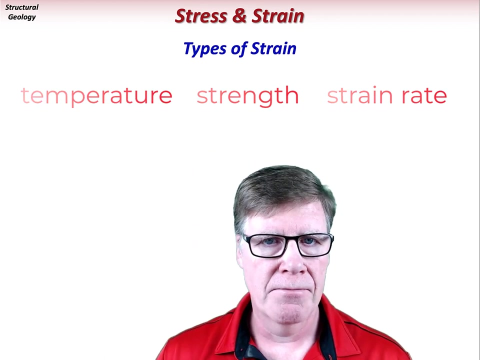 basic types of strain: brittle and ductile. Three factors that control the type of deformation include the temperature of the rocks, the strength of the rocks and the rate at which the rocks are being strained, also known as strain rate. Faults are geologic structures. 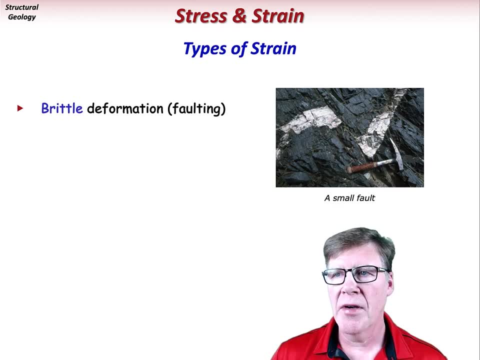 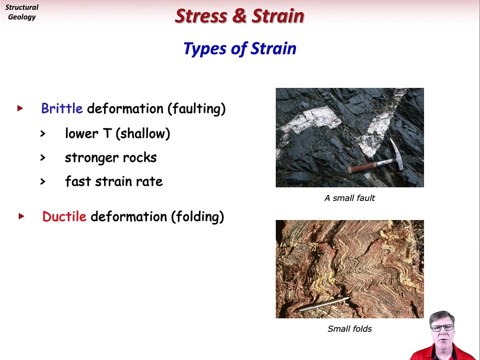 that represent brittle deformation. Brittle deformation typically occurs in rocks at lower temperatures, at more shallow levels in the crust. Stronger rocks also tend to deform in a brittle fashion. Finally, a relatively fast strain rate typically results in brittle deformation. Folds are geologic structures that represent ductile deformation- Ductile- 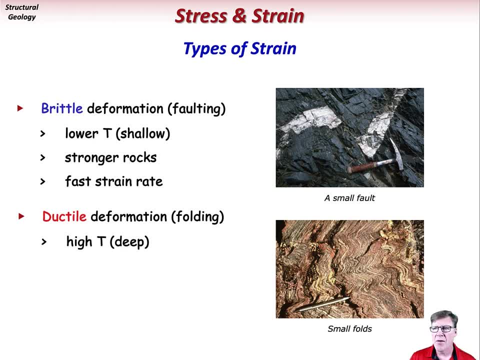 deformation occurs in rocks at higher temperatures found at deeper levels in the crust. Weaker rocks also tend to deform in a ductile fashion. Finally, a relatively slow strain rate results in ductile deformation. Note, ductile deformation is often referred to as plastic deformation, Not that it has anything to do with real plastic. 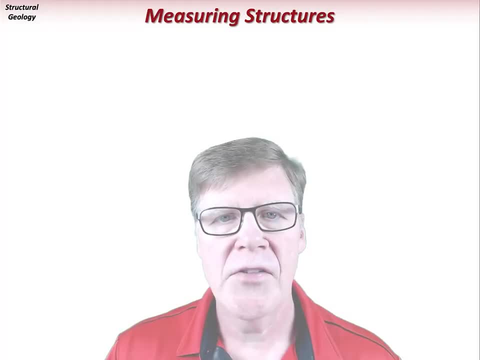 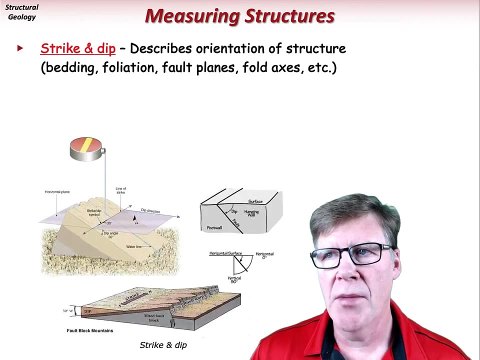 though. A structural geologist identifies geologic structures in the field. Strike and dip are measurements that describe the orientation of geologic structures, whether it's bedding, foliation or the structure of the rock. A structural geologist identifies geologic structures in the field. Strike and dip are measurements that describe the orientation. 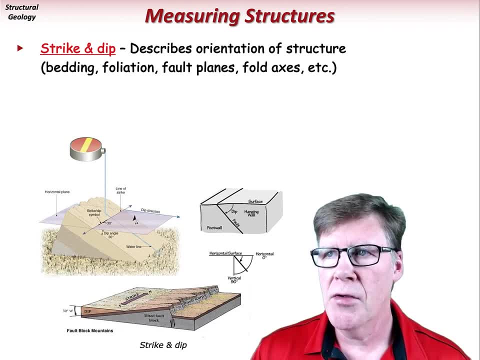 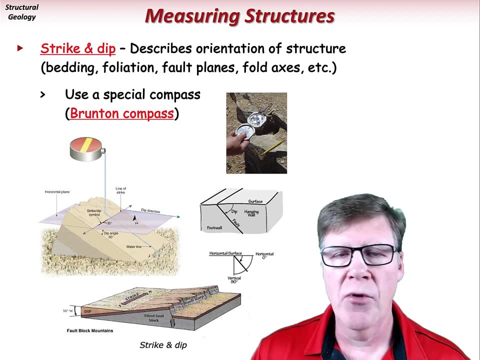 of geologic structures. Note: ductile deformation occurs in rocks at lower temperatures. In structure ma부� Vul criterion two: weéntime Dip health isпurtty easy to visualize. For it we note the diection of dip, which can be divided into a degree or delete pattern. 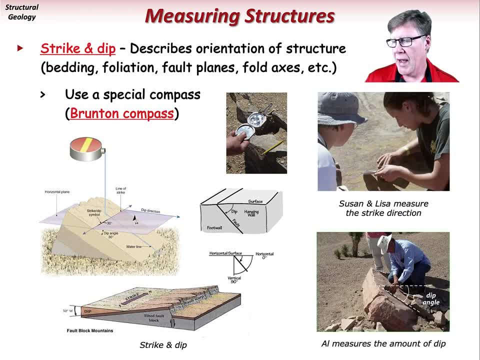 and 90 being vertical. Al is measuring the dip of bedding at a tilted sandstone outcrop. Not sure what the dip direction is here somewhere off to the right, but it looks like the dip angle is about 30 degrees from horizontal. 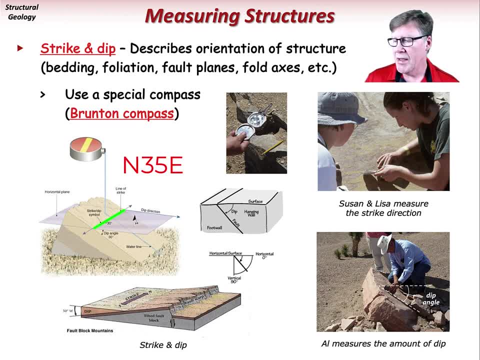 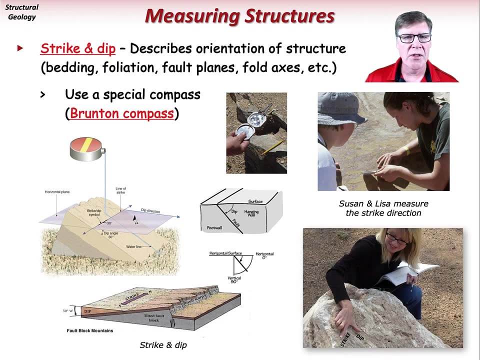 Strike is the compass direction of the line formed by the intersection of the feature, whether it's bedding or foliation or whatever, with an imaginary horizontal surface. It's a little more abstract to visualize than dip, so it helps that the strike direction is always 90 degrees or at right angles to the dip direction. 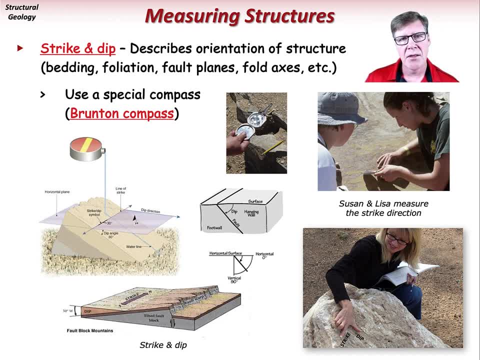 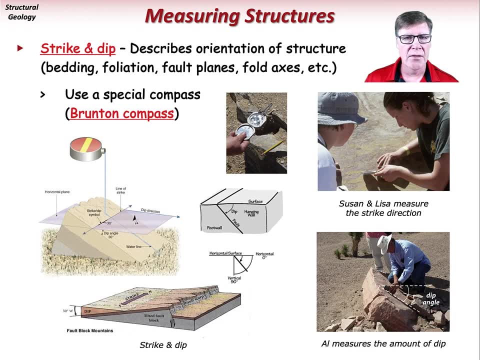 So if you know the dip direction you can easily figure out the strike direction. Susan and Lisa are measuring the strike of bedding of the Shinarump Conglomerate in St George, Utah. Once the strike and dip are measured, the two measurements are combined and written. 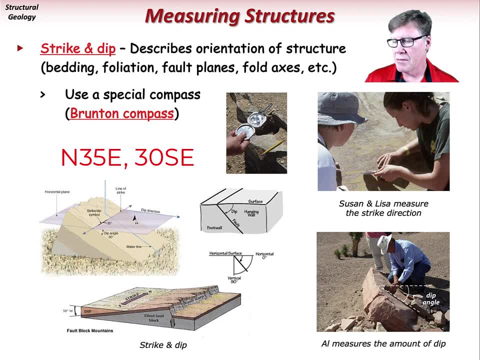 something like this: this North 35 East, 30 Southeast. North 35 East is the direction of strike and 30 Southeast is the amount and direction of dip. This information is crucial in documenting deformed layers and geologic structures, so that we can identify the geologic structures, make structural interpretations. 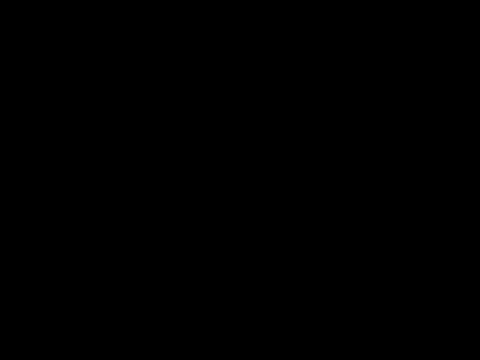 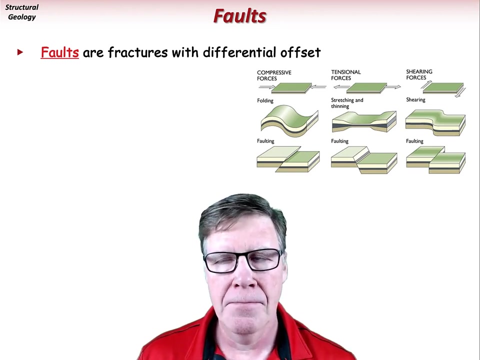 construct geologic maps, etc. Faults are deformational features that are essentially fractures with differential offset. Faults form under brittle conditions from any type of stress, tension, compression or shear. There are three basic types of faults with offset that may be oriented anywhere. 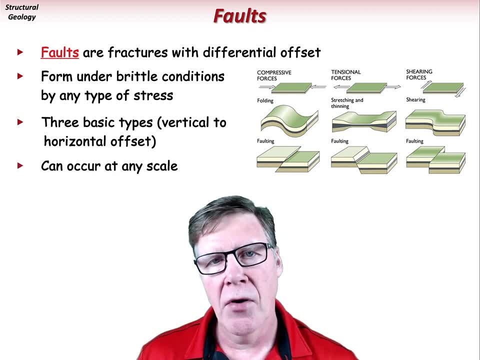 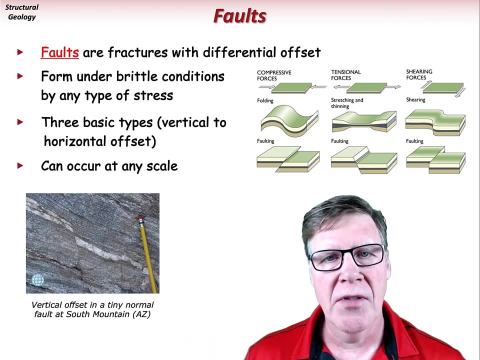 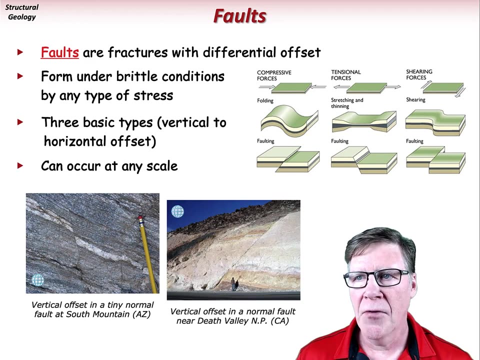 from vertical to horizontal. They can also occur at any scale, microscopic to mountain sized. Here a small fault with millimeters of offset is present in the Estrella Nice at South Mountain in Phoenix, Arizona. This fault is located along California Highway 178 at Resting Springs Pass, just east of Death. 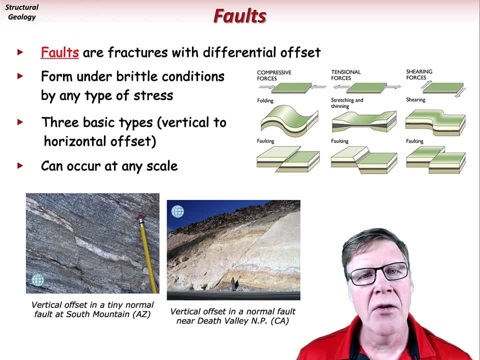 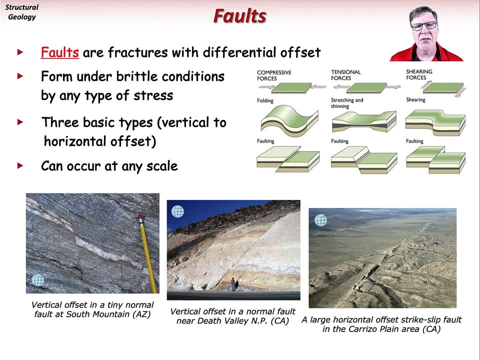 Valley National Park. This fault has a few meters of offset. Finally, the mighty San Andreas Transform Fault, here seen in the Carrizo Plain area, has over 500 kilometers of offset and is also the boundary between two different tectonic plates. 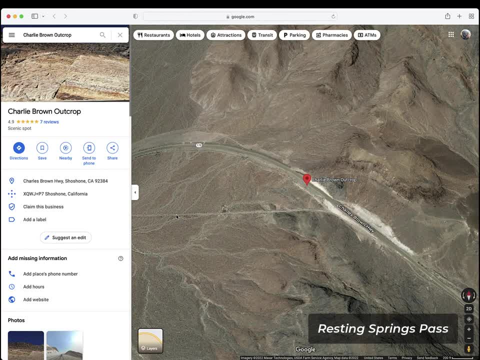 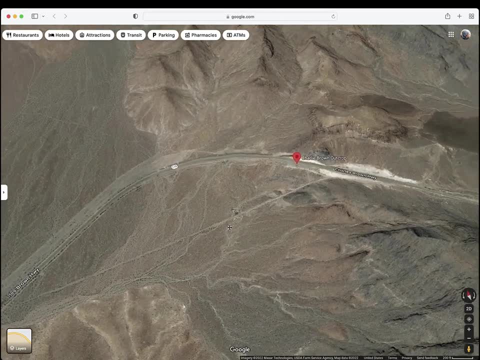 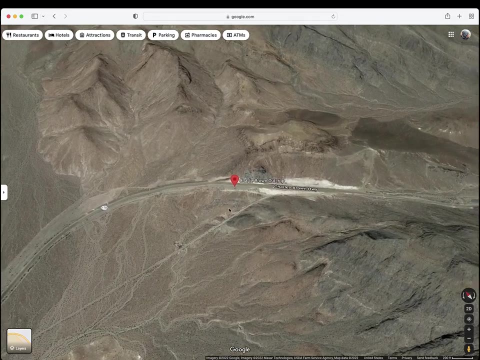 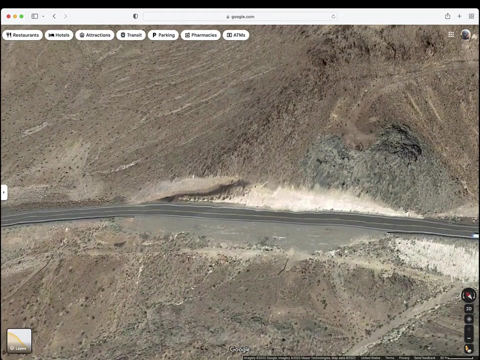 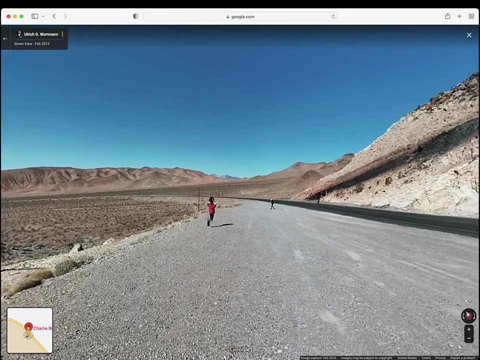 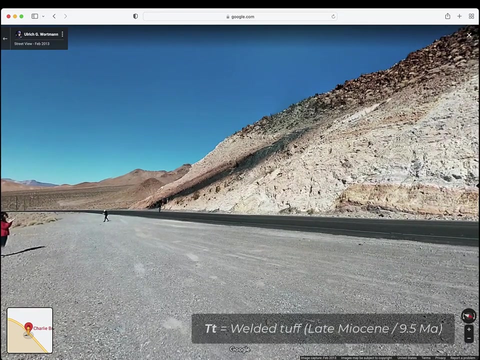 Resting Springs Pass is located in the Mojave Desert near the Nevada-California state line. Along California Highway 178, near Death Valley National Park, is a spectacular road cut of 9.5 million year old welded tuff, The black layer. there is part of the welded tuff, as is the cream colored unit. 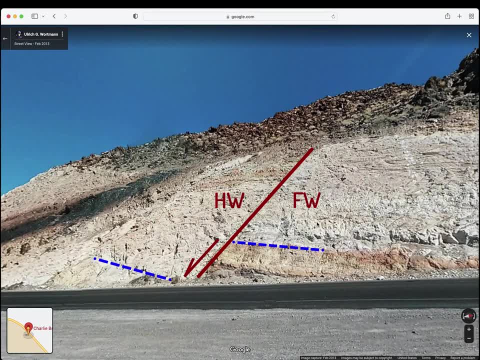 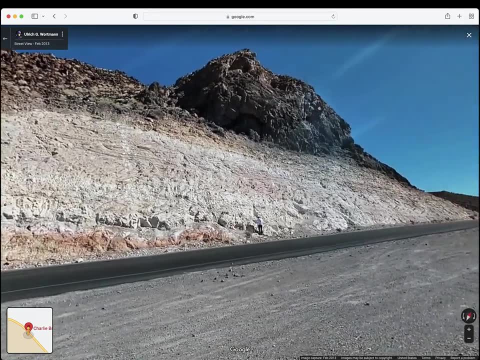 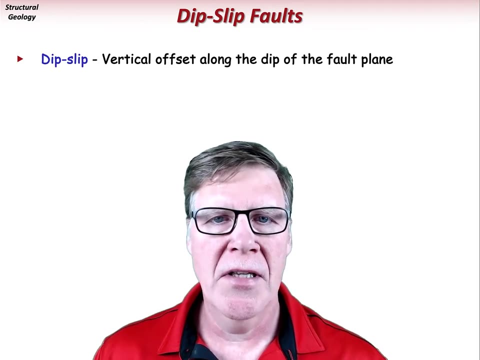 Several normal faults offset the tuff with west side down displacement. The fault is located in the upper plate of the fault plane. This fault is located into a strip of wood where the tuff is not visible. Dipslip faults are ones that have vertical offset along the dip of the fault plane. 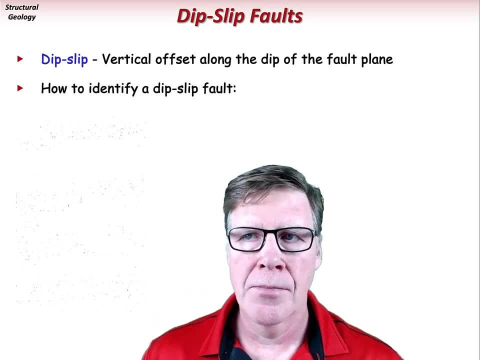 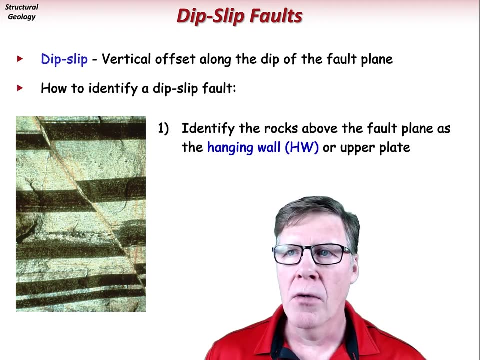 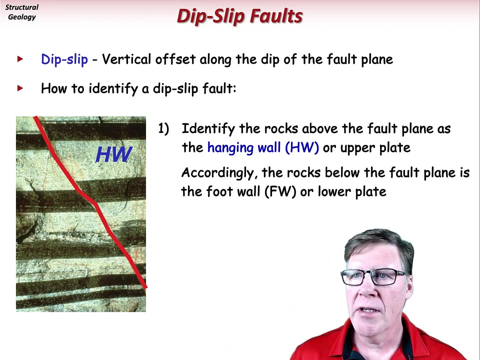 We can identify a dipslip fault in just a few steps. Once the dipslip fault is located, we can describe the part above the fault plane as the hanging wall. In really big fault systems, this may also be called the upper plate. Accordingly, the part below the fault plane is the hanging wall. 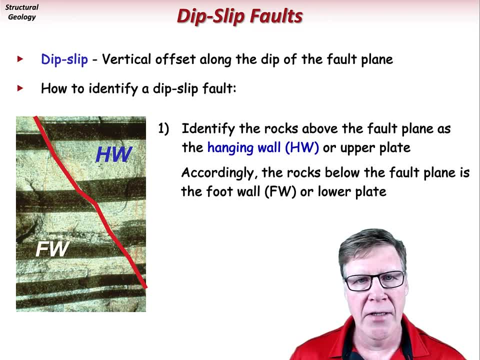 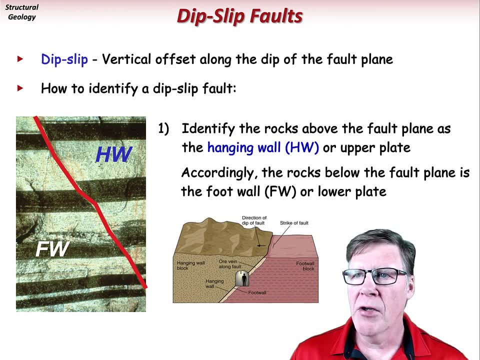 The fault space is located in the upper plate of the fault plane and is also called the upper plate is the footwall or lower plate in big faults. Hanging wall and footwall are older terms originally derived from underground mining operations. 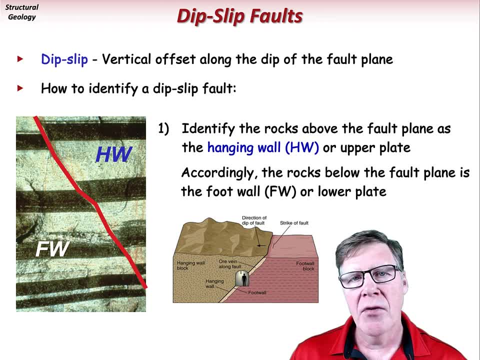 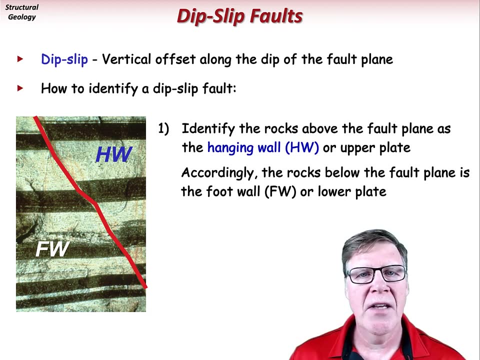 Ore bodies in their associated mining tunnels are often located along fault planes. In the tunnel, a miner can hang from the rocks above their head- thus the term hanging wall- and the rocks at their feet are part of the footwall. Once we have identified the hanging wall and footwall, 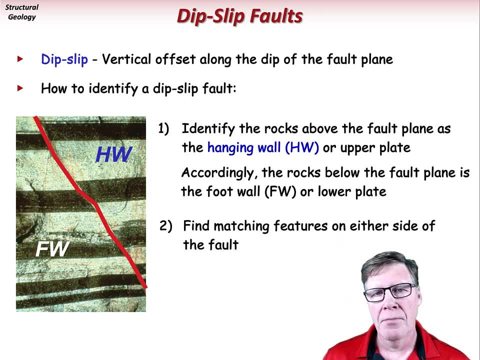 we need to find matching features on either side of the fault, commonly a distinctive bedding layer. From looking at the offset layers we next determine which way the hanging wall is moved up or down relative to the footwall. In the example here, the distinctive dark layers have been: 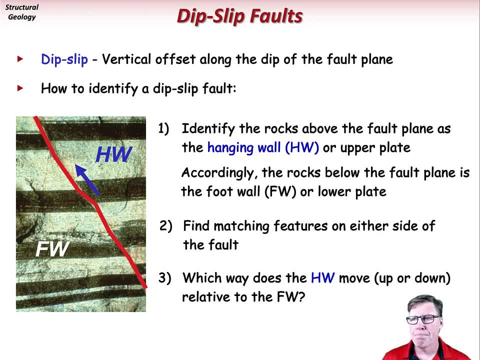 offset up on the hanging wall side. This enables us to more precisely identify the hanging wall and footwall. It should be noted that in many cases it is very difficult to find matching features on either side of a fault, so other means may be necessary to identify the fault. 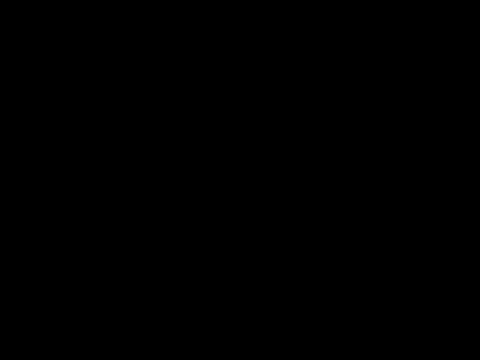 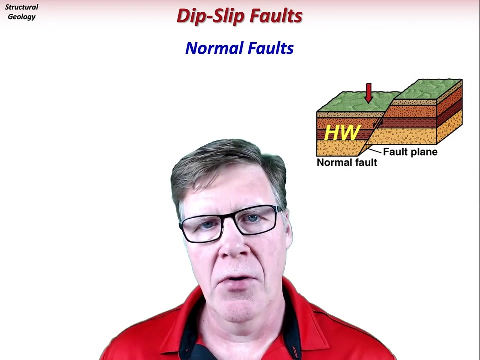 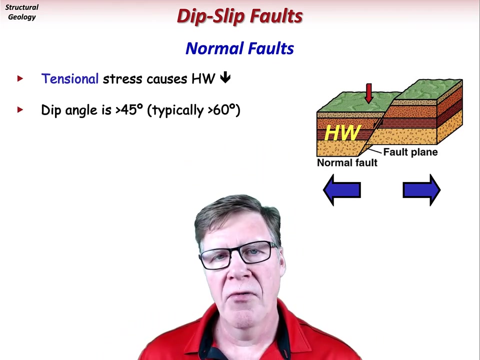 Normal faults are dip-slip faults, where the hanging wall is moved down relative to the footwall. These faults are caused by tensional stresses. The dip-and-slip fault is the fault that causes the hanging wall to move down, which causes the hanging wall to move up, The dip angle of most normal faults. 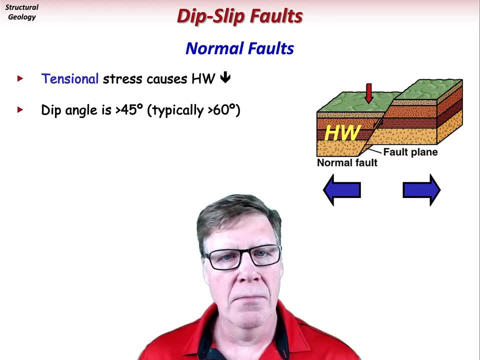 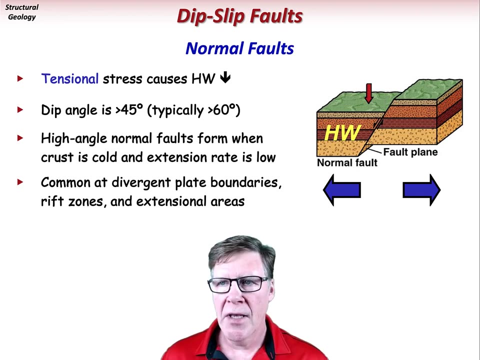 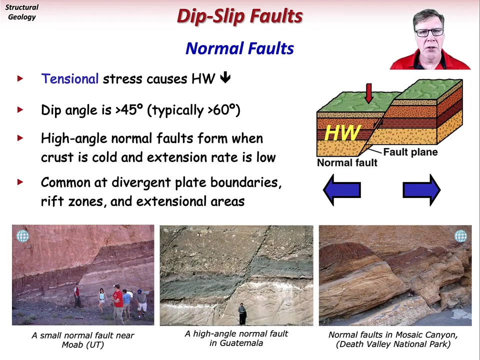 is greater than 45 degrees and commonly 60 degrees or more. These high-angle normal faults typically form where the crust is cold and extensional rates are low. Normal faults are common at divergent plate boundaries, rift zones and other extensional areas. At left is a small normal fault exposed. 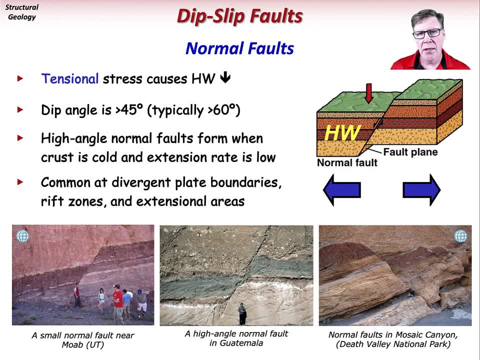 near the entrance to Arches National Park in Moab, Utah. At middle is a high-angle normal fault located in Guatemala, And at right are a series of small normal faults exposed in Mosaic Canyon in Death Valley National Park, Located along US Highway 191 near Moab Utah. 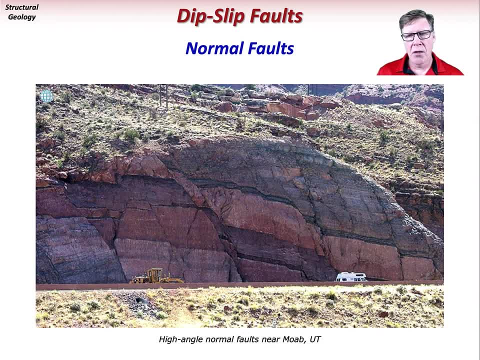 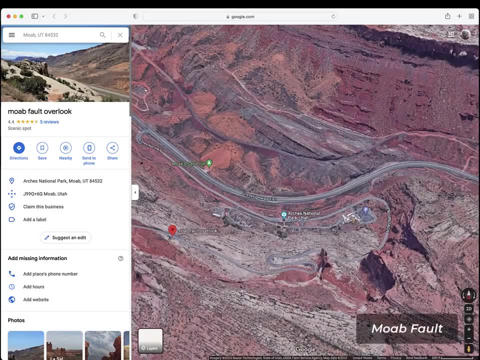 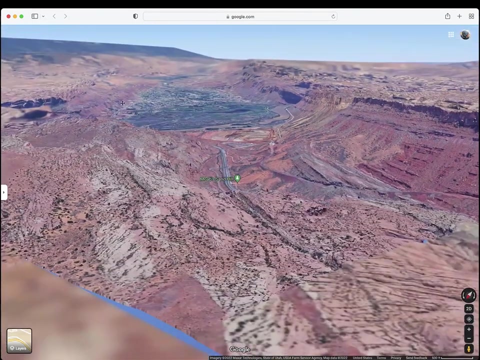 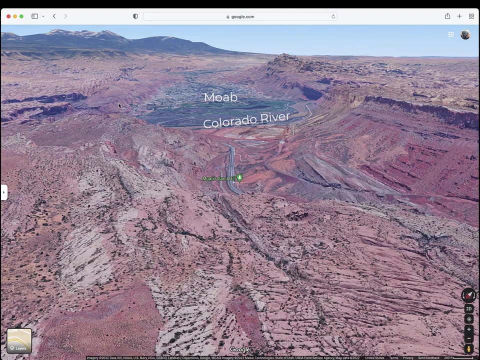 many high-angle normal faults are visible in this road cut, all formed from the same tensional stresses. Here we are at the northwest end of the Moab Valley, in the area around the entrance to Arches National Park, Looking southeast down the axis of the Moab Valley toward the Colorado River, Moab. 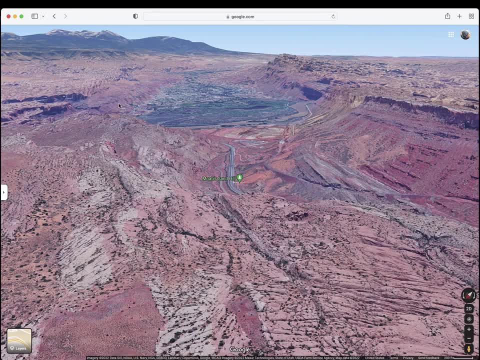 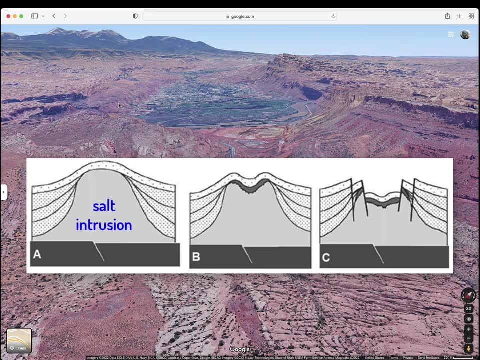 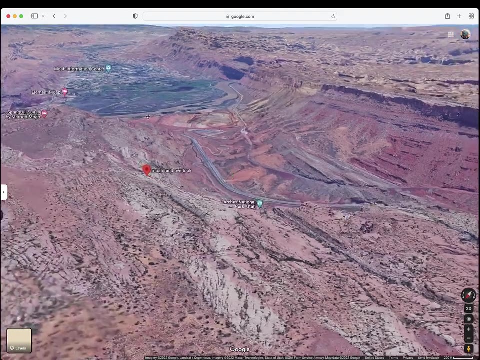 and the La Salle Mountains beyond The broad valley resulted from salt intrusion in Paleozoic and Mesozoic time and subsequent collapse caused by groundwater dissolution of the salt cap. The Mesozoic and Paleozoic sedimentary rocks have been arched up into a broad anticline. 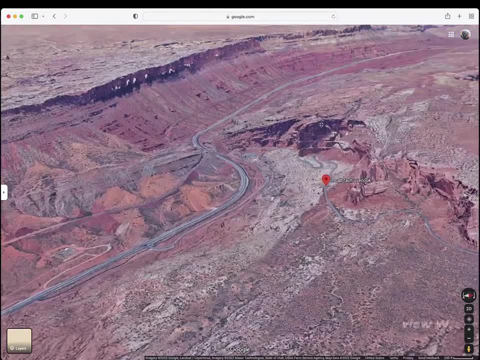 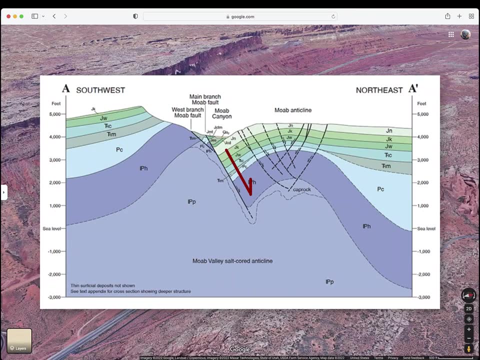 that has been cut by the Moab Fault, a large normal fault over 30 kilometers in length. Displacement of this fault is as much as 2,600 feet east side down. Vertical movement along the fault is not due to normal tectonics but salt tectonics from the 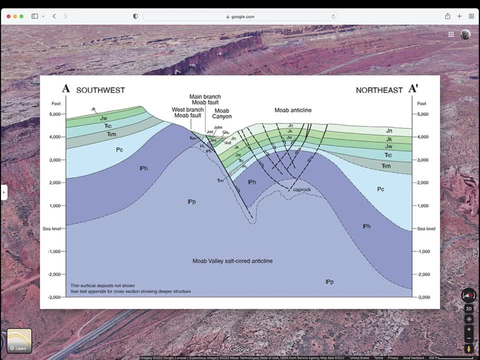 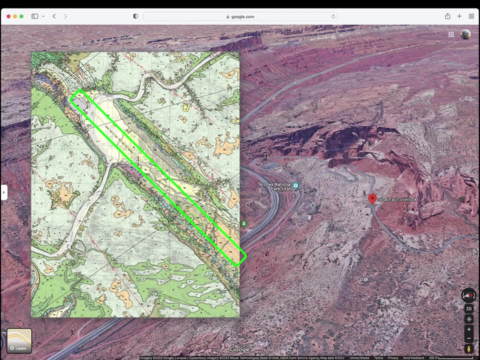 presence and movement of thick deposits of buried salt of the Pennsylvania Paradox Formation. Groundwater dissolution of the Paradox Salt is responsible for most of the displacement along the Moab Fault. The Moab Fault is largely buried beneath quaternary surficial sediments. 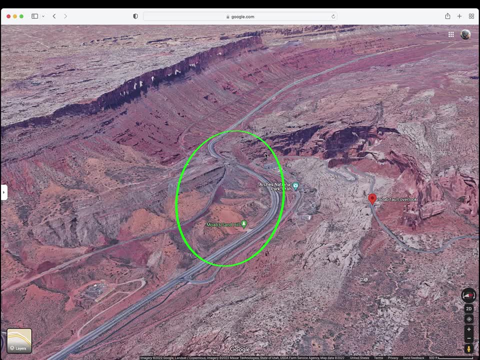 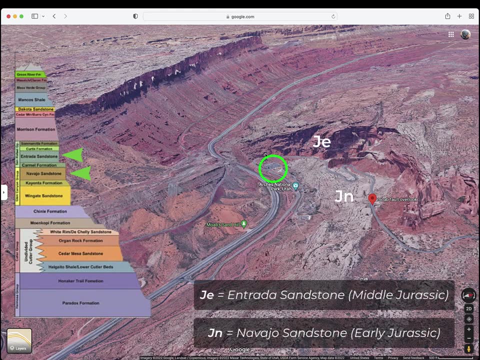 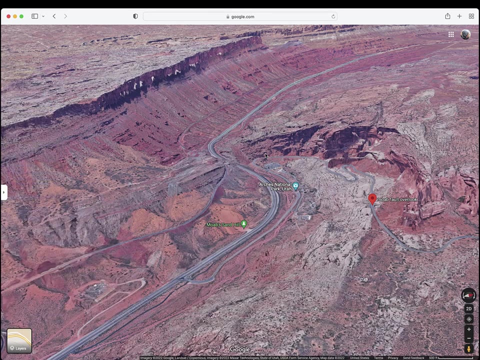 but is exposed in the area across from the entrance to Arches National Park. Here the Jurassic, Navajo and Entrata sandstones form the landscape around the park's visitor center, whereas older rocks are exposed in the cliffs to the west. This definitely means there's a fault in the area. 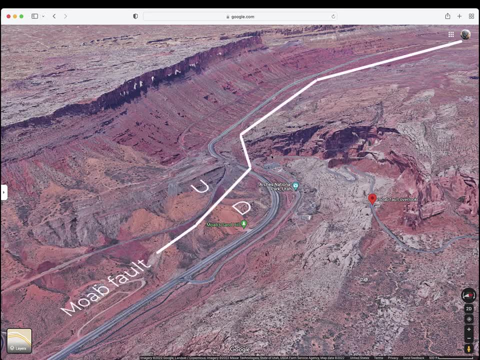 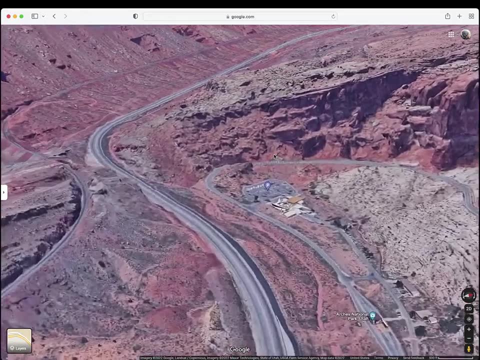 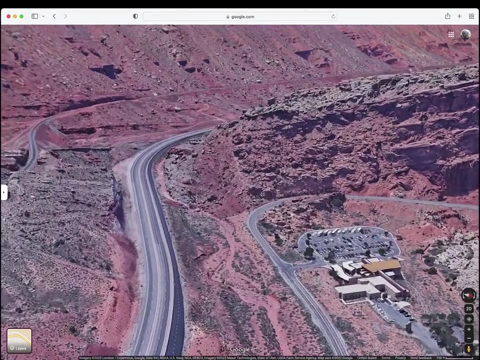 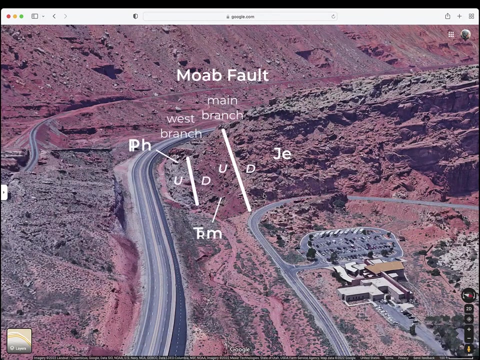 US Highway 191 more or less follows the trace of the Moab Fault expansions to the Moab Fault. Exposures of the Main Fault and the West Branch of the Moab Fault are located just west of the visitor center and across the highway. 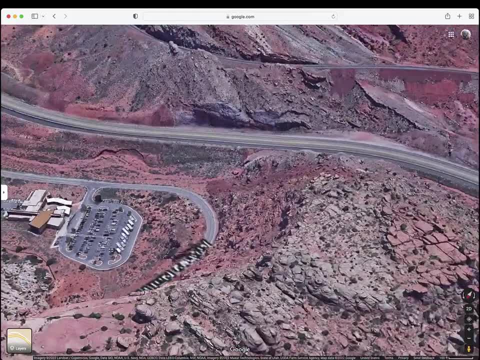 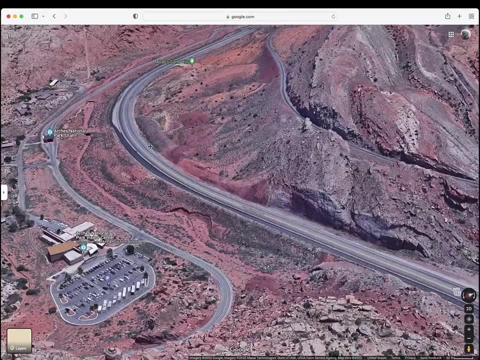 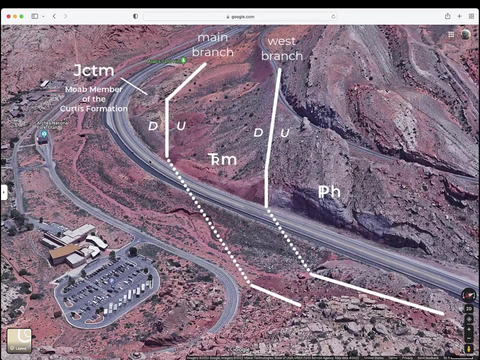 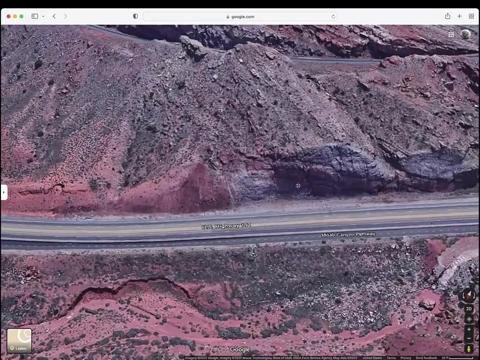 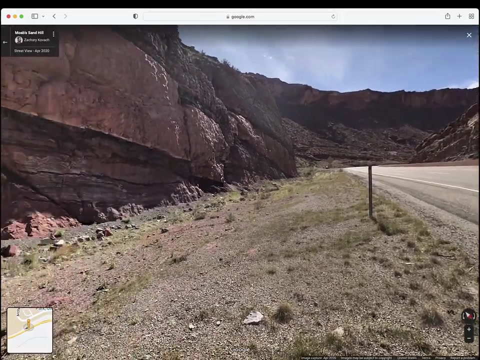 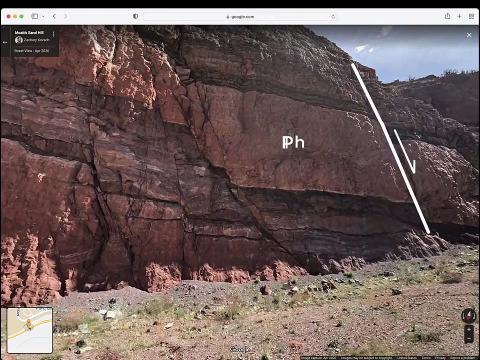 Several small normal faults are well exposed in the outcrop along the highway. Notice that the west side down movement sense on these smaller secondary faults is opposite that of the main fault which is east side down. These are called antithetic faults, common in areas of normal faulting. 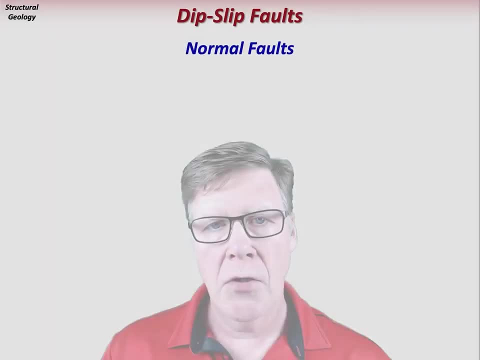 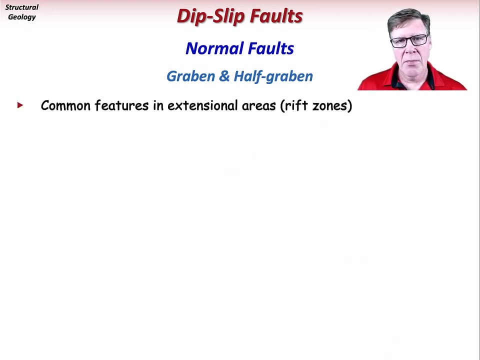 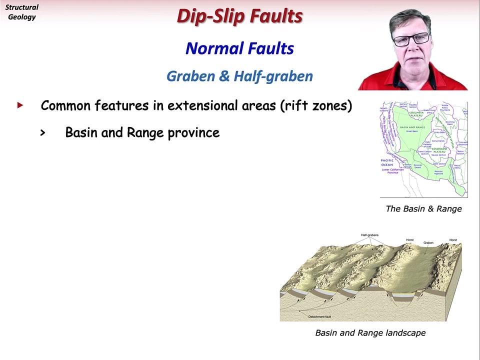 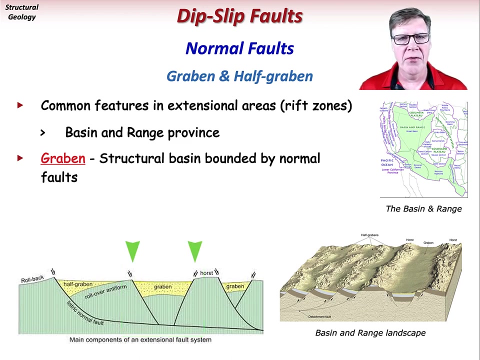 Grobben and half grobben are geologic structures common in extensional areas and rift zones. The basin and range province of the western United States and northern Mexico is a wide rift that includes many of these structures. A grobben is what we call a structural basin bounded by normal faults on either side. 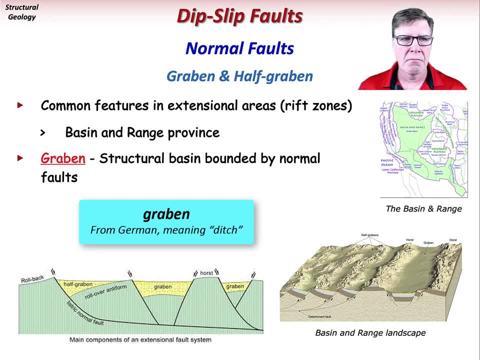 The word grobben itself is German for ditch, So if you really want to play the part, you can pronounce it graben. The hanging wall drops down relative to the footwall, often with little or no tilting. The resulting lower area, or grobben, typically fills with sediment eroded from the bordering. 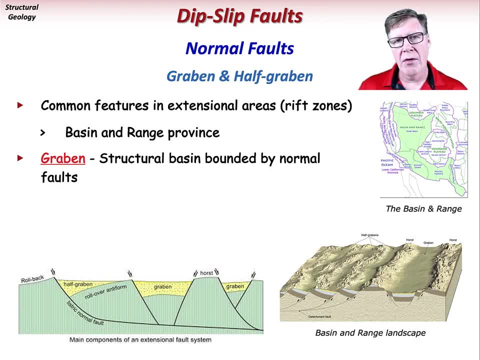 mountains in the footwalls. Indeed, these footwall mountains are called horse German for heap. The basin and range gets its name from the geology of these grobbens and horse. Many of the mountain ranges in the region are exposed footwall horsts and many of 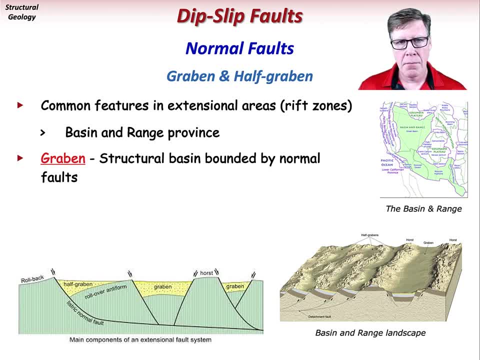 the basins are located in the grobben areas. A half grobben is a structural basin with a normal fault only on one side. This is analogous to a trapdoor. The normal fault in a half grobben typically forms above a curved or lystric fault. 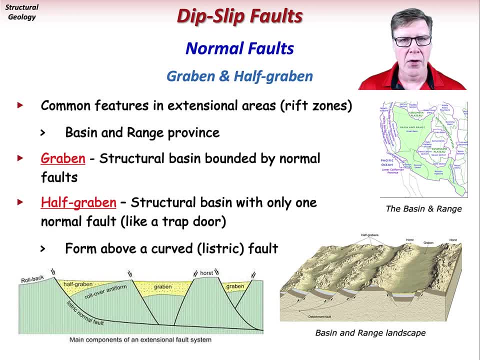 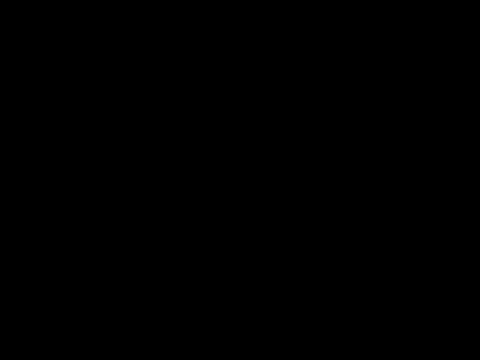 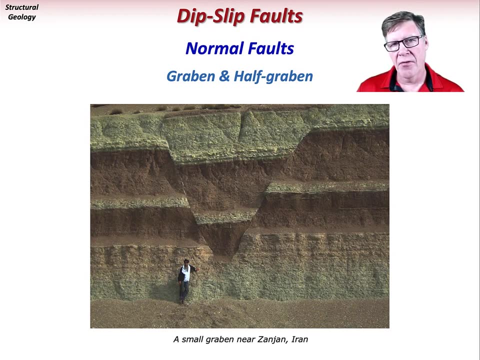 This causes the hanging wall rocks to become tilted towards the normal fault. Grobben and half grobben can form in the same areas. This is a view of some very distinctive layering, with small but extremely well preserved faults forming a grobben structure, and this is exposed near Zahan Iran. 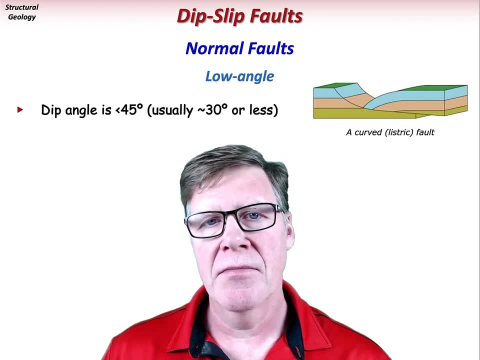 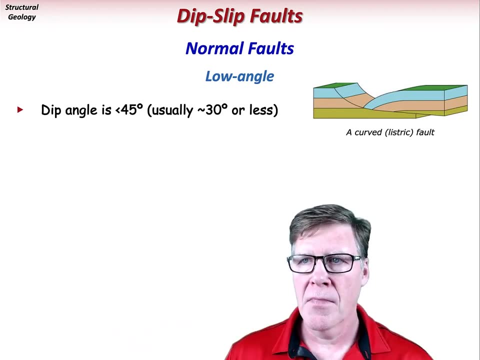 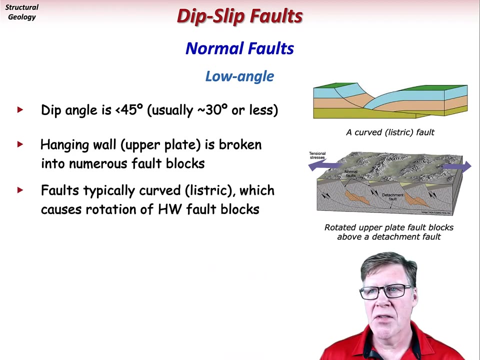 Some normal faults have dip angles less than 45 degrees and commonly less than 30 degrees. These are known as low angle normal faults. The hanging wall or upper plate is commonly broken into numerous fault blocks and since a low angle normal fault is typically curved, or lystric movement along the fault causes. 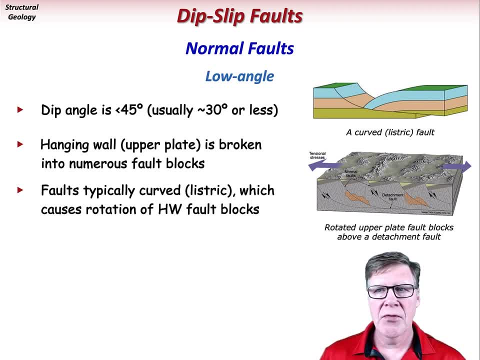 rotation of the hanging wall blocks, usually tilting them in the same general direction toward the fault plane. Large low angle faults are also known as detachment faults and are generally master faults with significant horizontal displacement. They are found in areas where the crust is relatively hot and the extensional rate is. 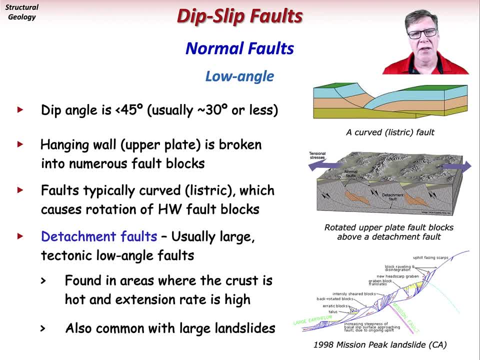 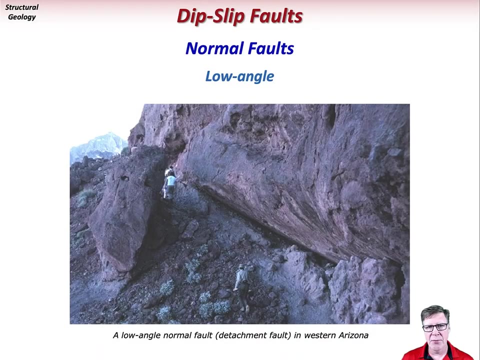 high Low angle faults are also common in large landslides and serve as the glide plane or décollement for the landslide mass. A great example is the 1998 Mission Peak landslide located north of San Jose, California. This is a low angle normal fault or detachment fault exposed in the buckskin- rawhide mountains. 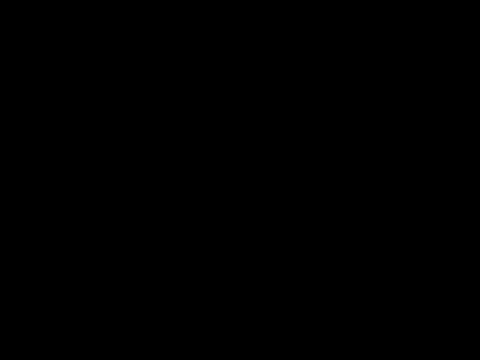 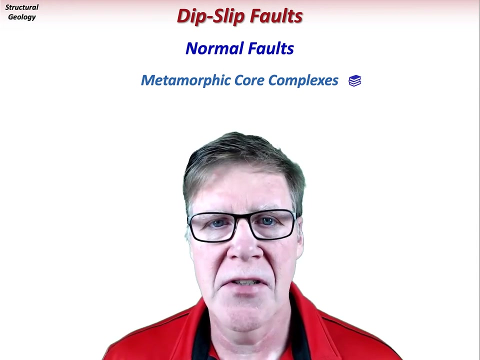 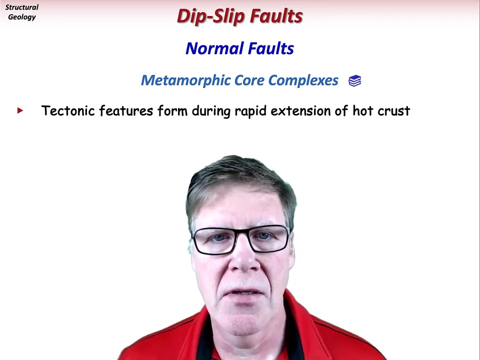 of western Arizona. Metamorphic core complexes are large extensional features first described relatively recently, in the early 1980s. These tectonic structures form during rapid crustal extension of relatively hot crust As movement proceeds along a large detachment fault. this is a low angle normal fault. 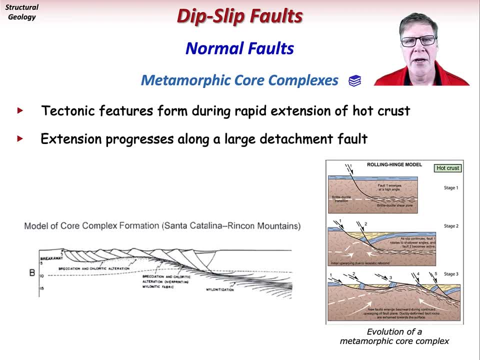 This is a low angle normal fault or detachment fault exposed in the buckskin rawhide mountains of western Arizona. The upper plate breaks up into separate fault blocks that rotate with continued extension. As the upper plate becomes progressively thinner, the deeper crustal metamorphic crystalline 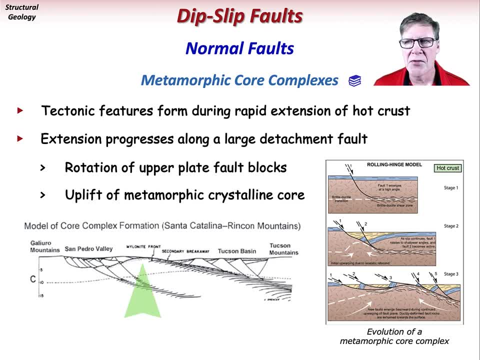 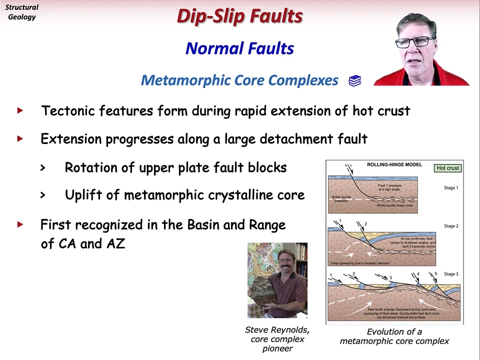 rocks of the lower plate begin to rise and eventually become exposed. Thus a metamorphic core complex is formed. Geologists like PJ Coney, George Davis and Steve Reynolds mapped and described these extensional tectonic features first recognized in the Basin Range province of California and Arizona. 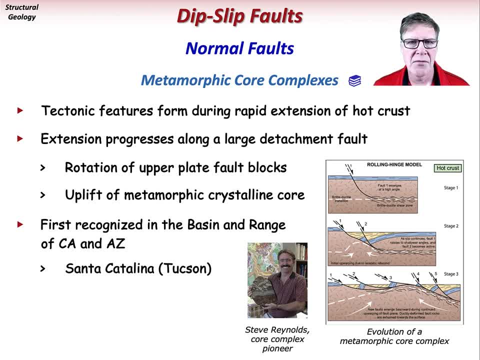 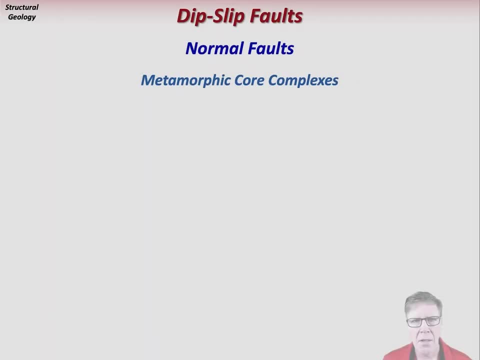 Significant localities stretch from the Santa Catalina Mountains of Tucson to the South Mountains of the Phoenix area, to the buckskin rawhide mountains of western Arizona, to the Whipple Mountains of southeastern California. This is a simple Steve Reynolds cross-sectional sketch of the South Mountains metamorphic core. 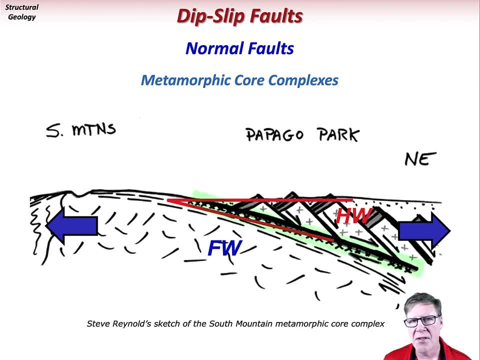 complex. The South Mountains detachment fault is the main low angle normal fault here. The South Mountains themselves represent the crystalline, igneous and metamorphic rocks of the lower plate that have now been exposed by extension. Belle Butte, Tempe Butte, the Papago Buttes, etc. are the exposed parts of the rotated 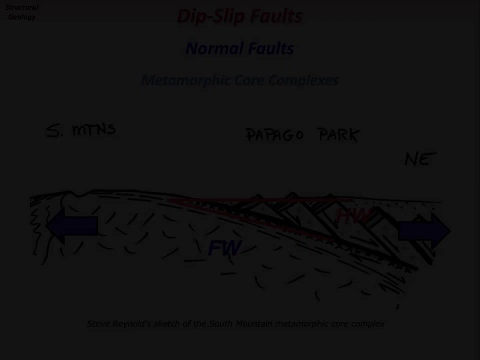 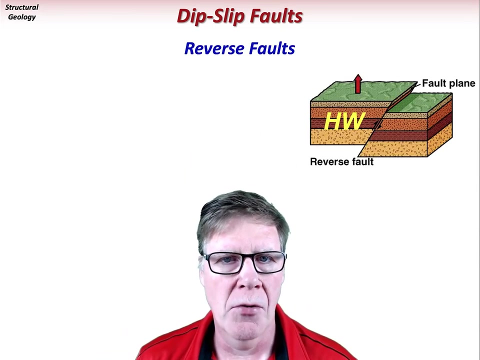 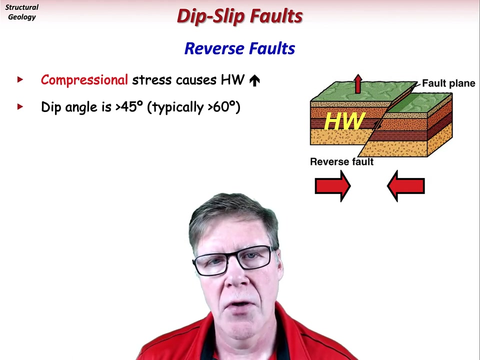 tilt blocks of the extended upper plate. Reverse faults are dip-slip faults, where the hanging wall is moved to the left side of the footwall and the wall is moved up relative to the footwall. These faults are caused by compressional stresses. The dip angle of most reverse faults is greater than 45 degrees and is commonly 60 degrees. 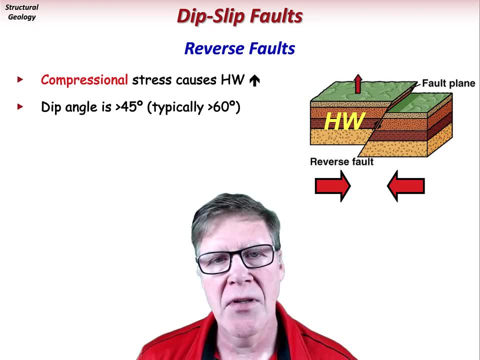 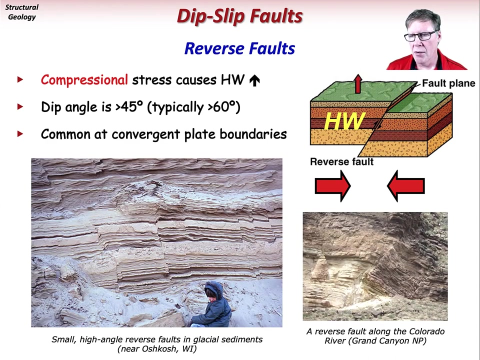 or more. These high angle reverse faults typically form when the crust is cold and the convergence rate is low. Reverse faults are common at convergent plate boundaries, including subduction zones and continent-continent collision areas. The image at left here shows several small reverse faults formed in glacial sediments. 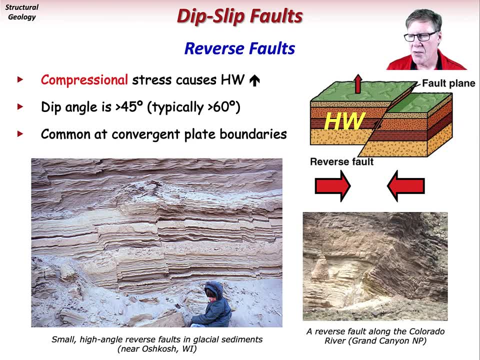 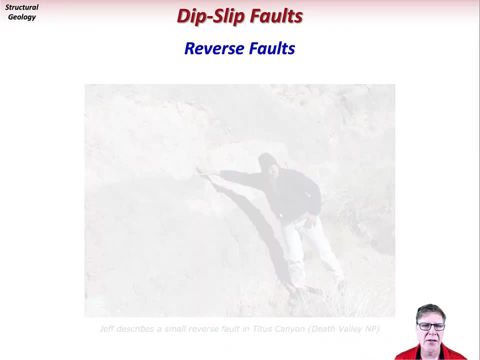 near Oshkosh, Wisconsin. At right is a small reverse fault related to the Monument Fold in the Ells Chasm area along the Colorado River. in Grand Canyon National Park, In Titus Canyon of Death Valley National Park. Jeff describes a small reverse fault to our 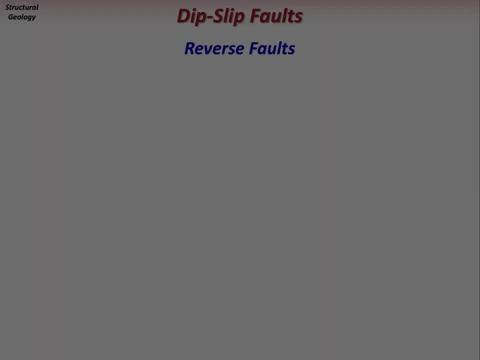 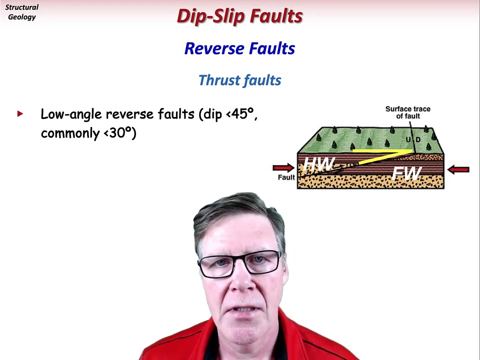 group. Some reverse faults have dip angles less than 45 degrees and less than 30 degrees. These are called thrust faults. These faults form when the rate of tectonic convergence is high and involve an upper plate moving up and over a lower plate. 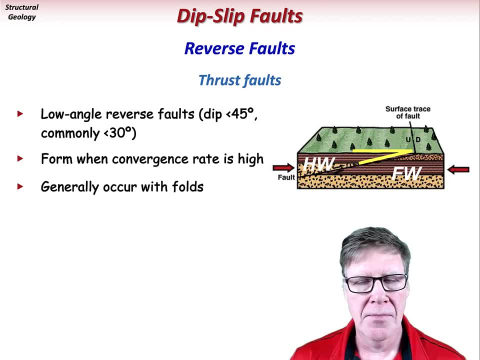 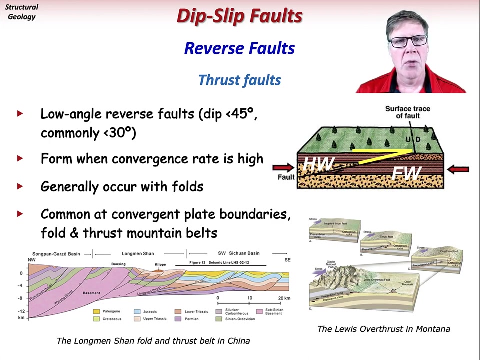 Thrust faults commonly accompany the formation of folds. Thrust faults are common at convergent plate boundaries, In some mountain belts, known as fold and thrust belts. tectonic compression creates a complex network of folds and folds. Typically, a basal master thrust fault forms and serves as the glide plane or décollement. 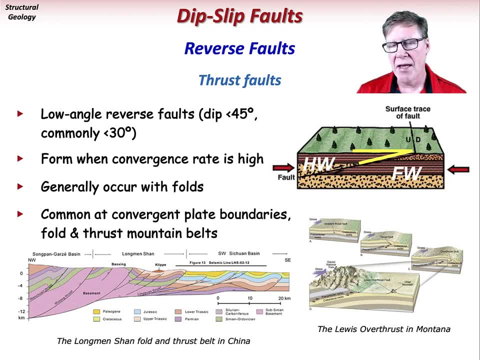 for the upper plate. These master faults can have significant horizontal displacement. Smaller reverse faults and thrust faults commonly extend upward from the basal thrust to the upper plate. Classic fold and thrust belts are found in the Rocky Mountains and Appalachian Mountains of North America, the Alps, the Zagros Mountains of Iran and in China, to name a few places. 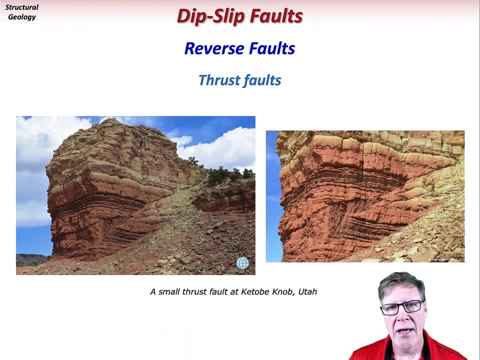 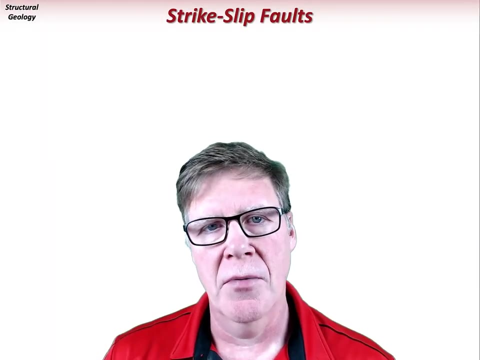 This is an example of a super well-exposed thrust fault at Katobi Knob in the San Rafael Swell area of central Utah. In the image on the right note the human for scale. Strike-slip faults are different from dip-slip faults in that shear stress causes mostly. 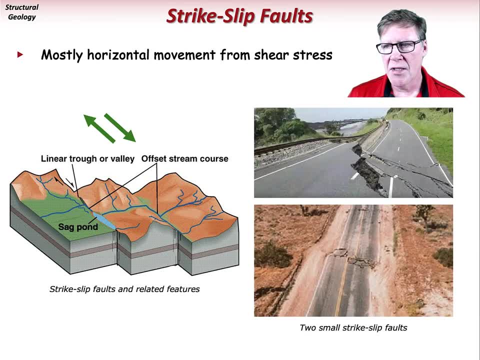 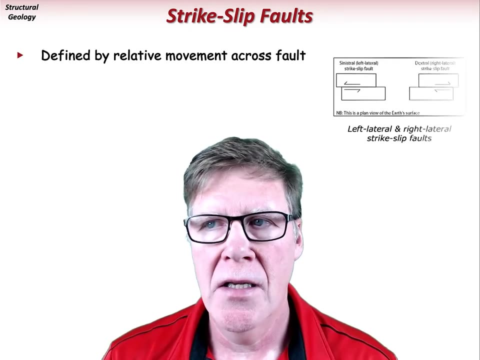 horizontal movement along the strike of the fault, not the dip of the fault. Strike-slip faults are usually nearly vertical, so there's really no hanging wall or footwall. Two varieties of strike-slip faults can be defined by the relative movement between fault. 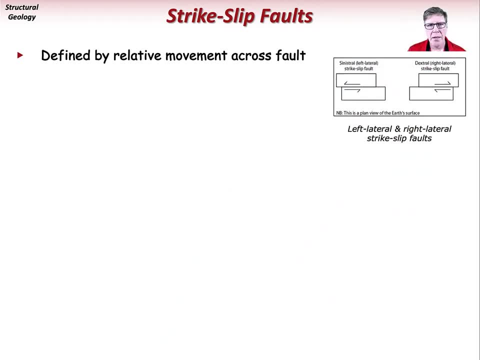 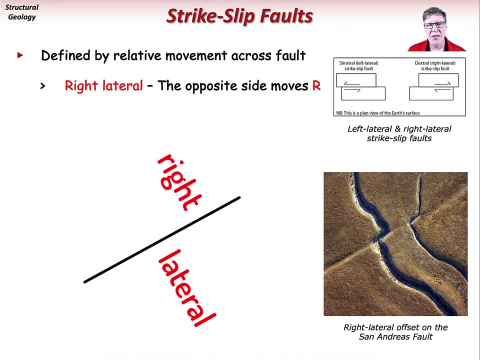 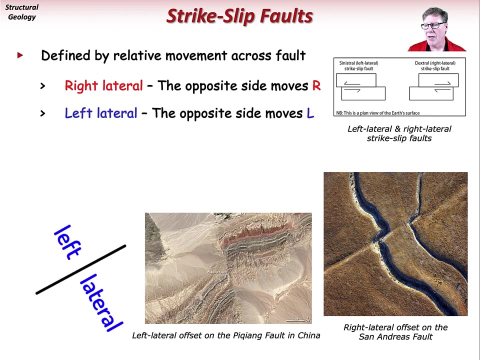 blocks. A right lateral strike-slip fault is one where the opposite side of the fault moves to the right. The San Andreas fault in California has a right lateral movement sense. Conversely, a left lateral strike-slip fault is one where the opposite side of the fault 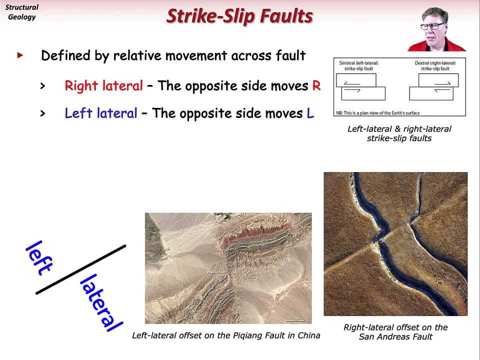 moves to the left. The Peking fault in northwest China has a left lateral movement sense. Strike-slip fault in the Peking region is an example of a right lateral strike-slip fault are common at transform boundaries and strike-slip faults that form the boundary between two tectonic 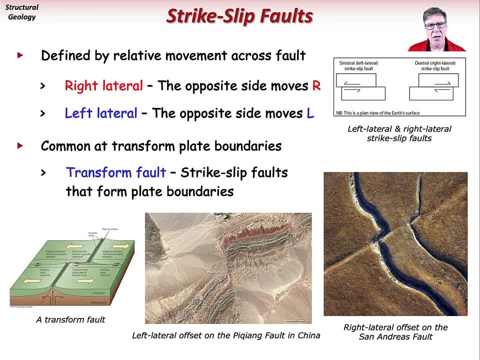 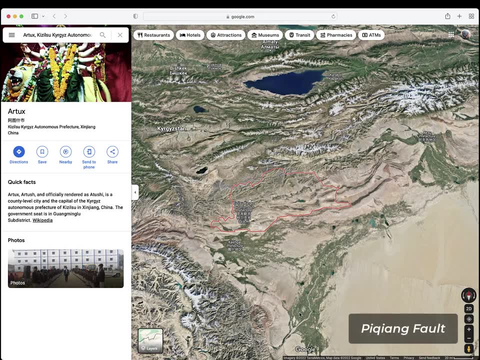 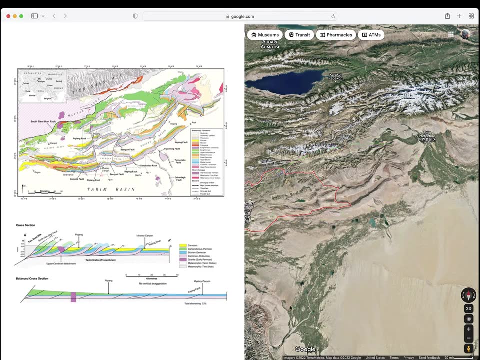 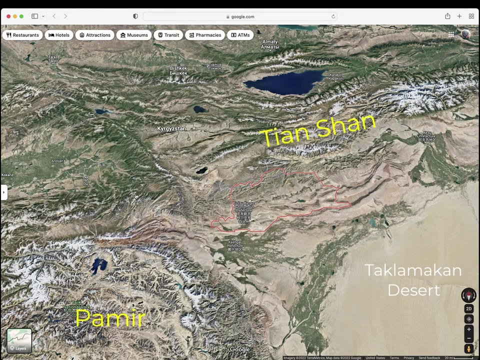 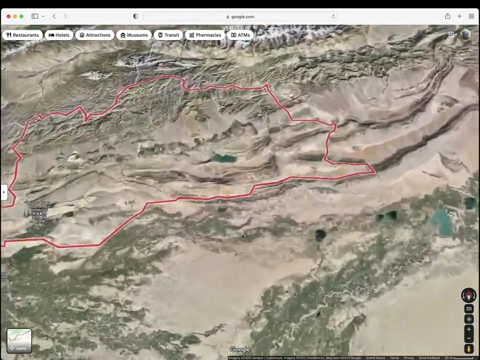 plates are known as transform faults. These commonly offset mid-ocean ridge segments. The Pikiang Fault is a northwest trending left lateral strike-slip fault in the Keping Shan Thrust Belt in northwest China. This area lies between the Tian Shen mountains to the north and the Takamakan desert to the south. 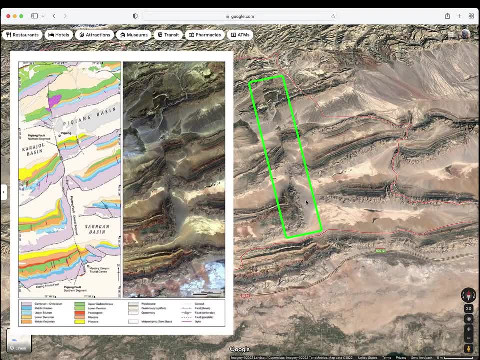 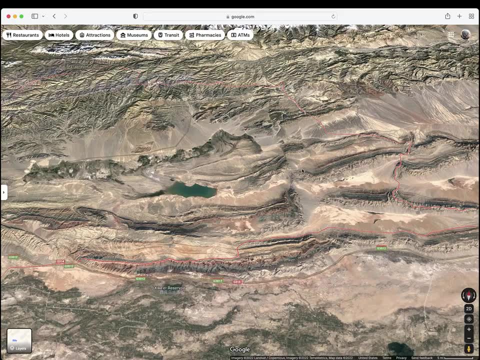 This strike-slip Fault is more than 70 kilometers in length and may have originated as a normal fault in the Permian, but was rescheduled, reactivated as a strike-slip fault during the middle to late Cenozoic, related to the Himalayan orogeny. 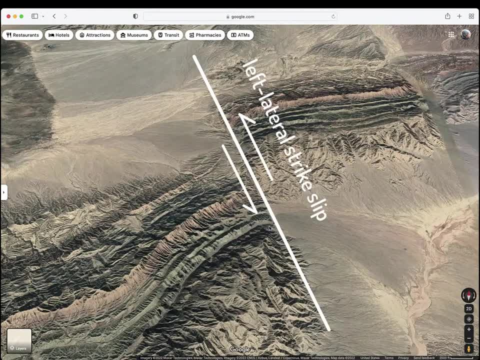 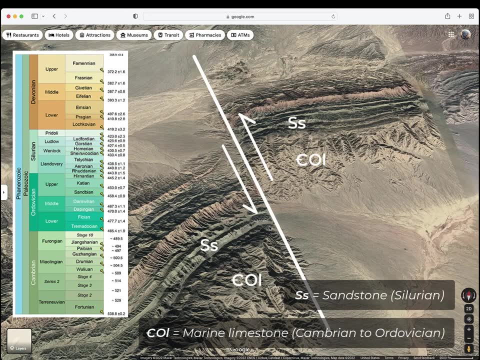 The rock units of note here include the older cream-colored Cambrian to Ordovician marine limestones, greenish Silurian marine sandstones, and the top of the sequence is made up of reddish Devonian fluvial sandstones. 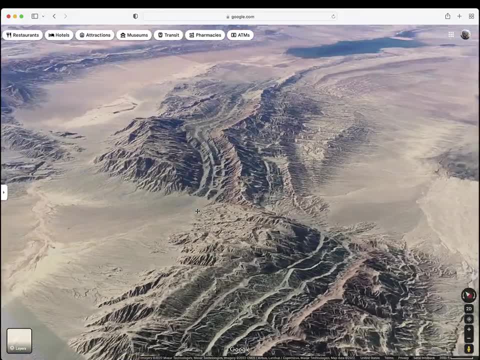 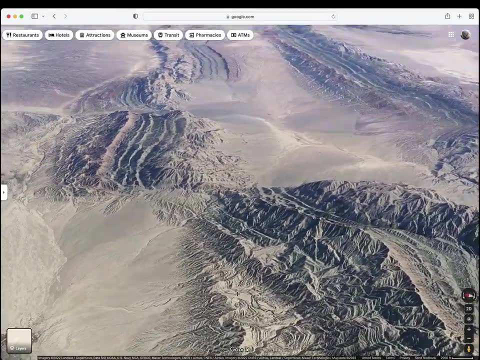 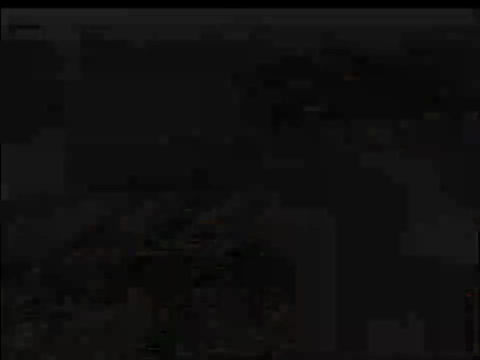 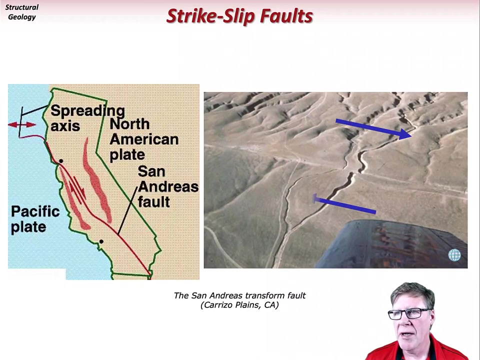 The San Andreas fault is a famous example of not only a strike-slip fault, but also a transform fault, because it forms the boundary between two tectonic plates. Specifically, the San Andreas fault is a famous example of not only a strike-slip fault. 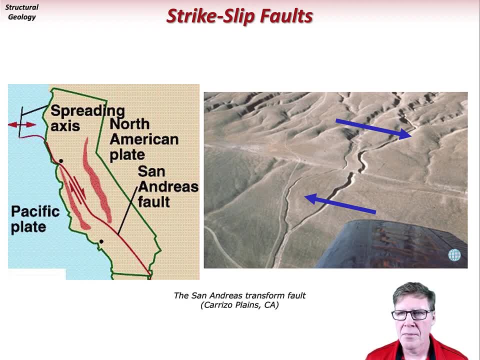 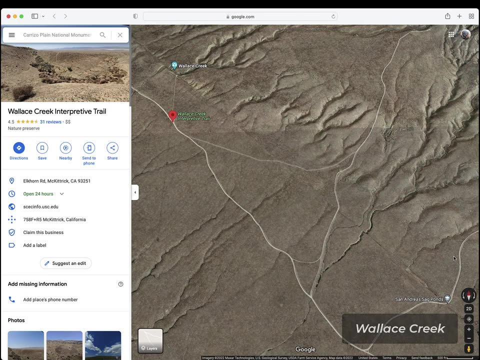 but specifically the Pacific and North American plates. And right here is the Wallace Creek area of the Carrizo Plain in south-central California. This is the Wallace Creek area of the San Andreas fault. It's a rather famous locality that shows the offset along the fault. 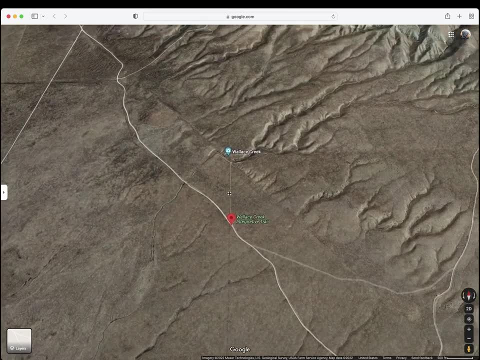 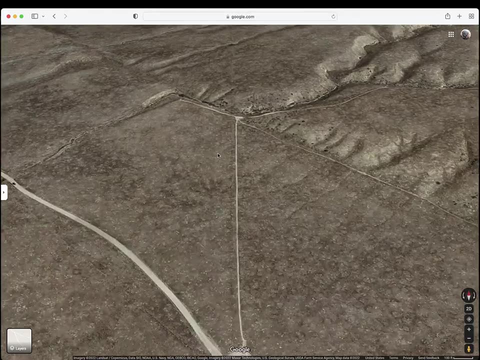 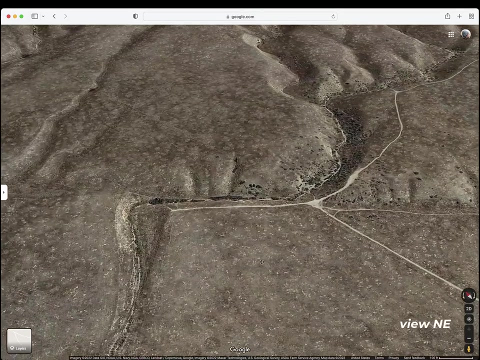 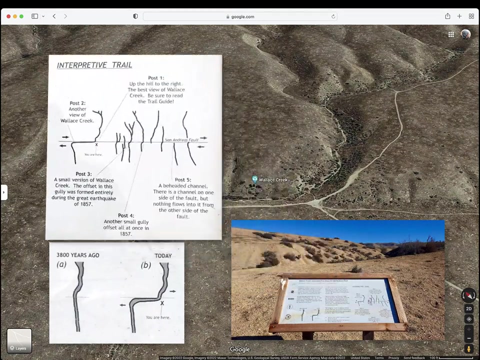 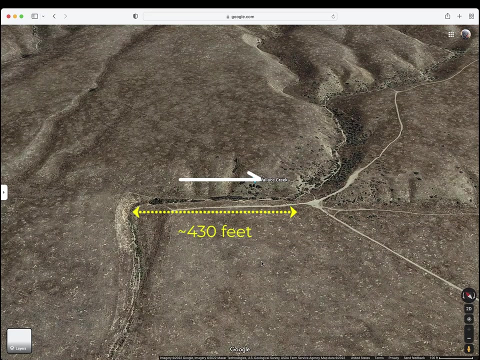 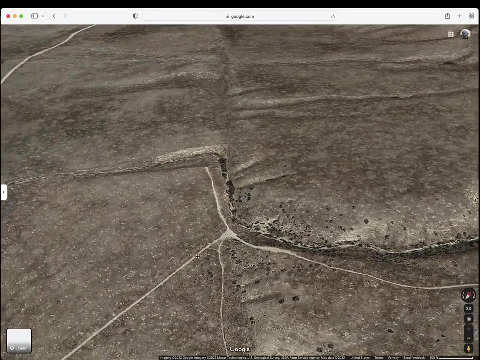 And right here is the Wallace Creek area of the Carrizo Plain in south-central California. The offset is about 430 feet here at Wallace Creek. During the 1857 magnitude 7.9 Fort Tohono earthquake alone, the San Andreas fault here moved about 30 feet. 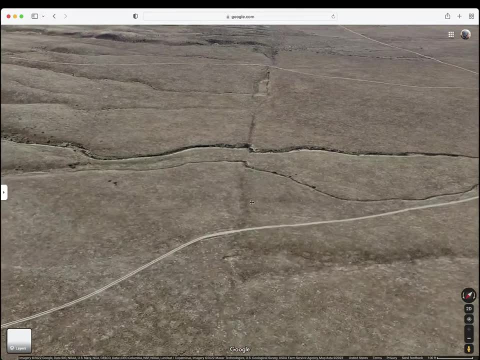 And right here is the Wallace Creek area of the San Andreas fault. During the 1857 magnitude 7.9 Fort Tohono earthquake alone, the San Andreas fault here moved about 30 feet. And right here is the Wallace Creek area of the San Andreas fault. here moved about 30 feet. 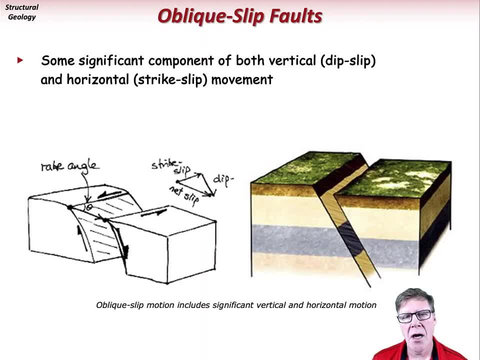 Oblique-slip faults are those with some significant component of both vertical and horizontal movement. These faults may be difficult to discriminate from dip-slip and strike-slip faults. Their identification largely depends on having good exposures along the fault. A joint is a joint. 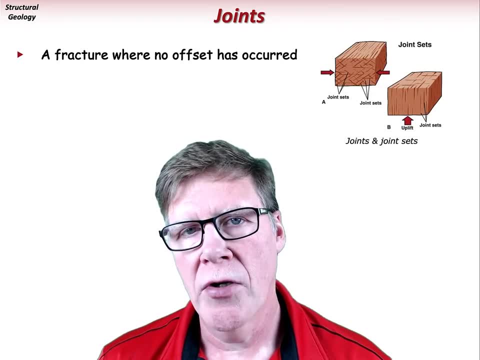 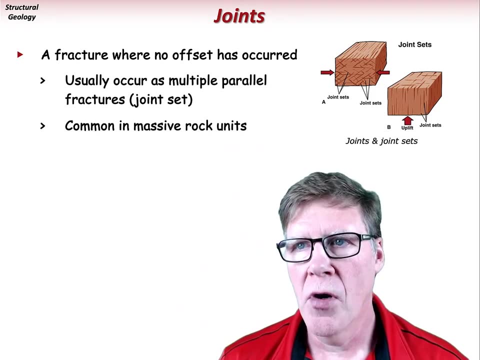 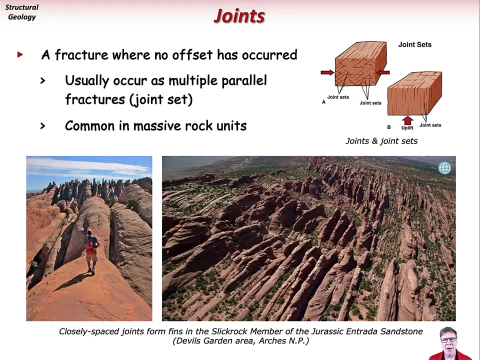 is a geologic structure represented by a fracture where no offset has occurred. Multiple parallel joints make up a joint set which commonly form in massive, compositionally homogeneous rocks. For example, the slick rock, member of the Entrada sandstone is a massive sandstone in Arches National Park. This unit hosts a dominant joint set that is: 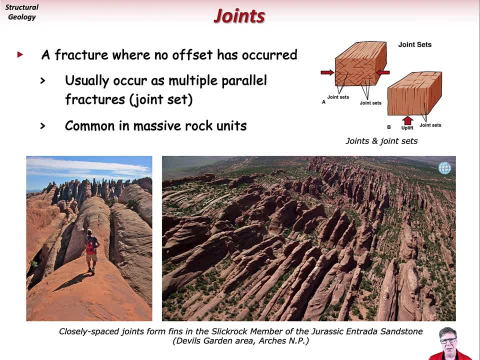 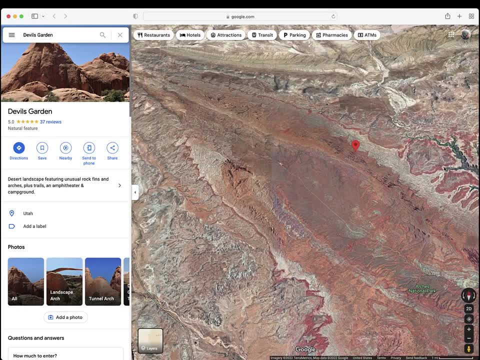 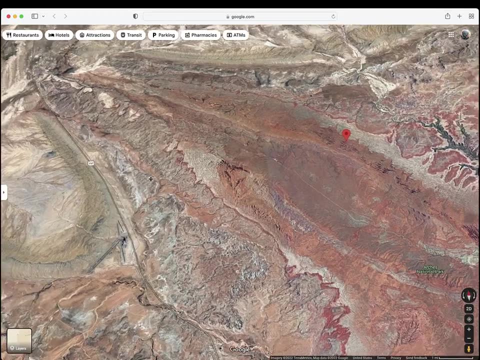 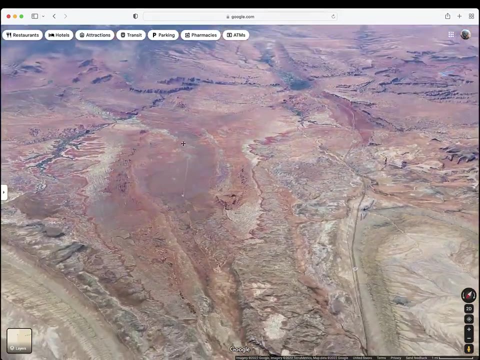 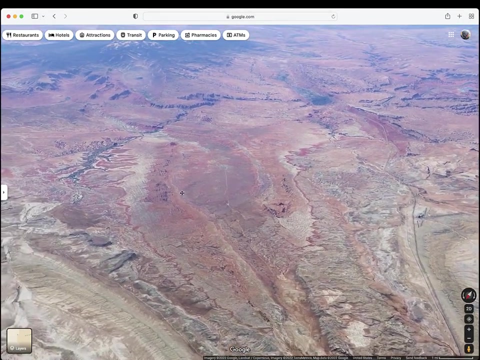 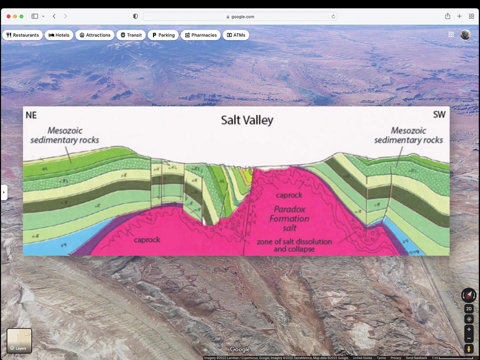 eroded into prominent fins and even arches in some locations. This is the Salt Valley area of Arches National Park. Here, mesozoic sedimentary rocks were long ago arched up into a northwest-trending anticlinal structure due to the movement of the deeper paradox formation: salt mass. 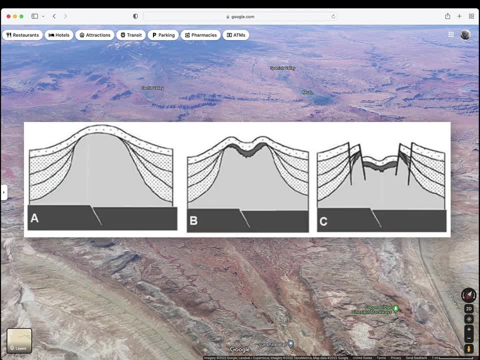 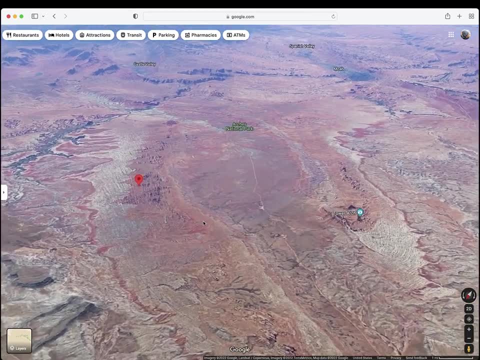 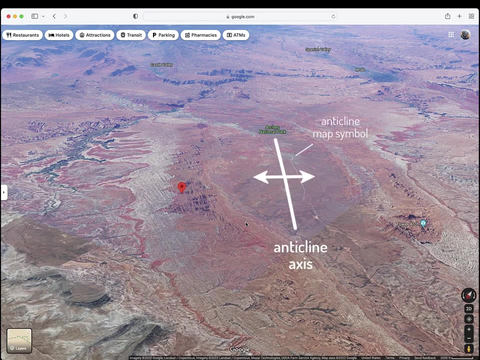 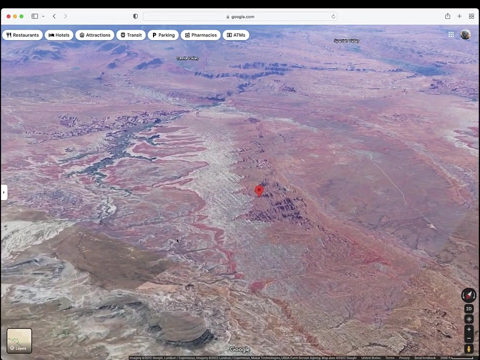 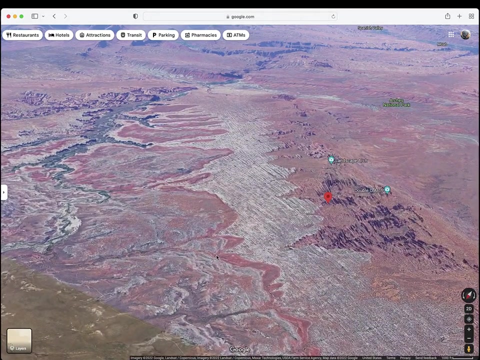 Subsequent dissolution of the salt along the crest of the anticline formed normal faults and created the Salt Valley Graben. The mesozoic rocks along the flank of the anticline are highly jointed as a result of the salt tectonics. 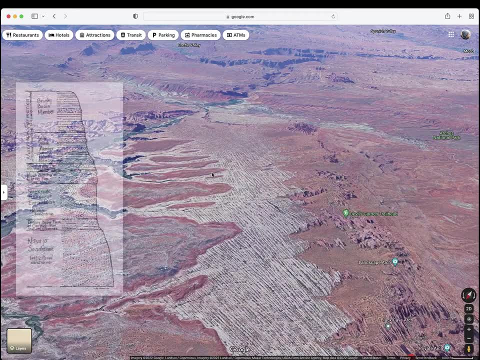 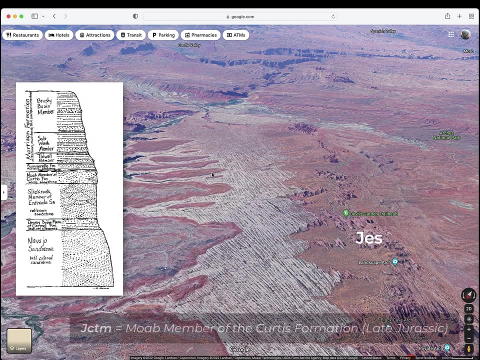 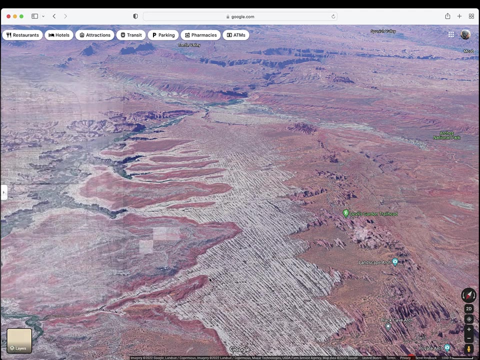 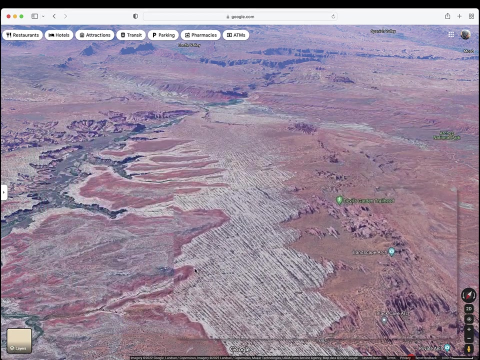 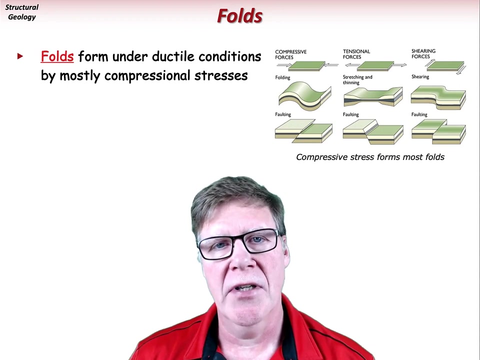 Seen here from right to left are the reddish rocks of the slick rock, member of the Entrada sandstone, And the cream-colored Moab, member of the Curtis formation. Folds are deformational features that form under ductal conditions and mostly from compressional stress. There are many different types of folds. 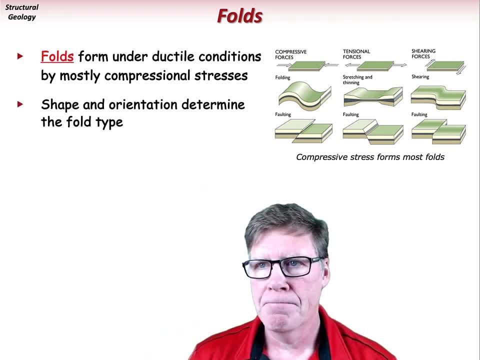 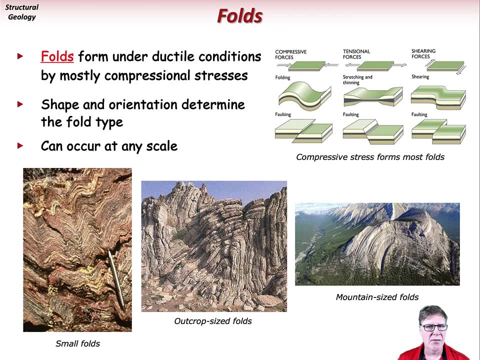 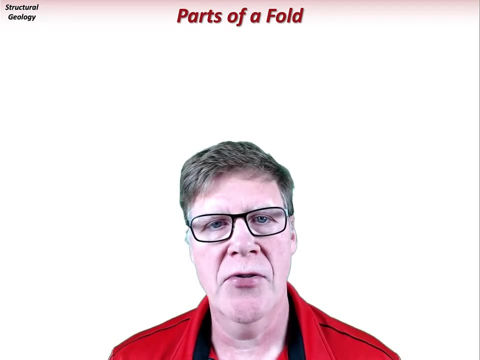 each different in their own form, Each distinguished by its shape and orientation. Folds can occur at any scale, from microscopic to hand-sample outcrop and even mountain-sized. A couple important parameters are used to describe the geometry of all folds. 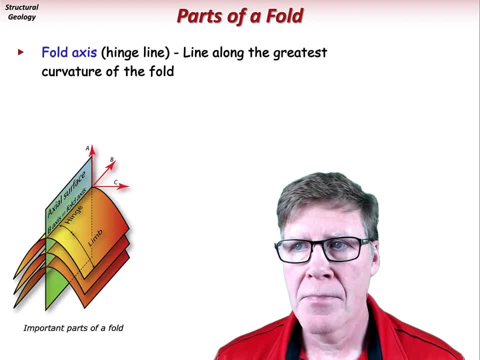 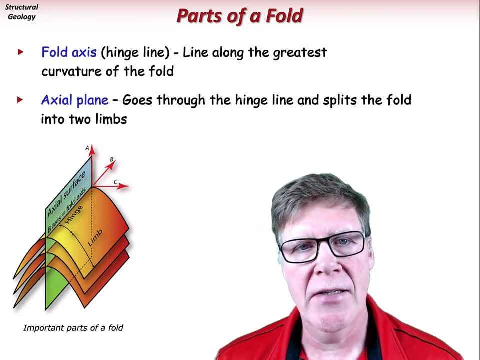 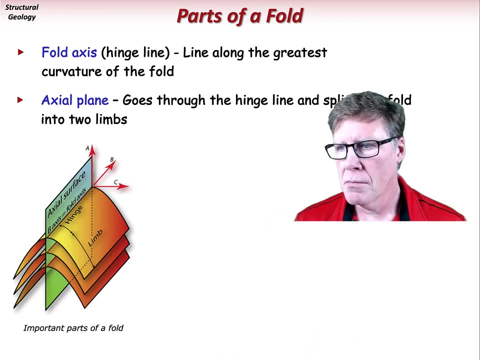 The fold axis, also called the hinge line, is the line that trends along the greatest curvature of the fold. The axial plane is an imaginary plane that goes through the fold axis and splits the fold into two equal parts called limbs. The axial plane may be vertical, horizontal or inclined at any intermediate angle. 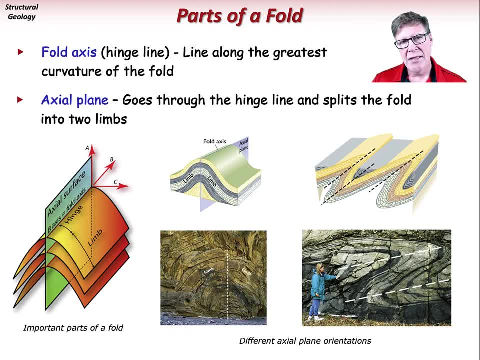 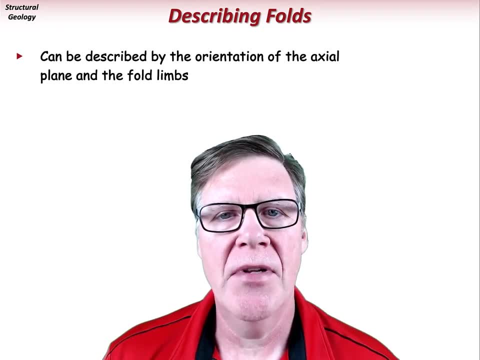 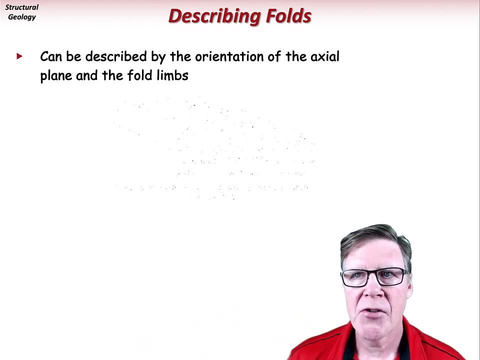 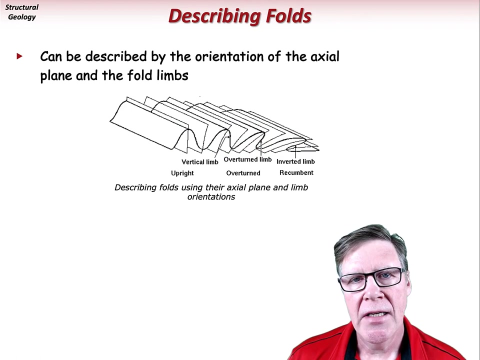 The recumbent folds shown at lower right. this image is one of my favorites. Important parameters that describe different folds are the orientations of the axial plane and the fold limbs. Axial plane orientations can range from vertical to inclined to nearly horizontal. Accordingly, the dip of each fold limb changes as well. 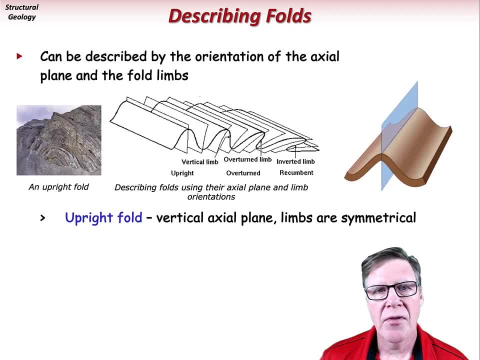 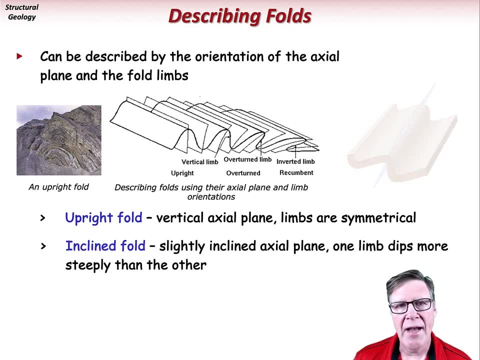 In an upright fold, the axial plane can be vertical, with the fold limbs symmetrically dipping away from the axial plane. An inclined fold is one where the axial plane is slightly inclined, with the forward limb having a steeper dip than the other. 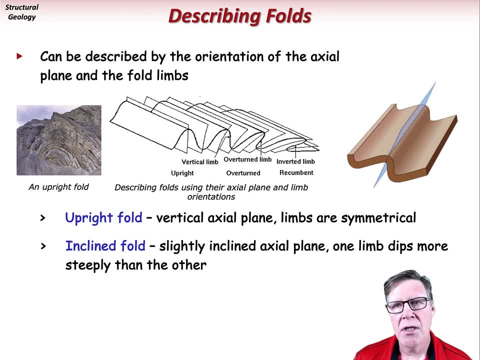 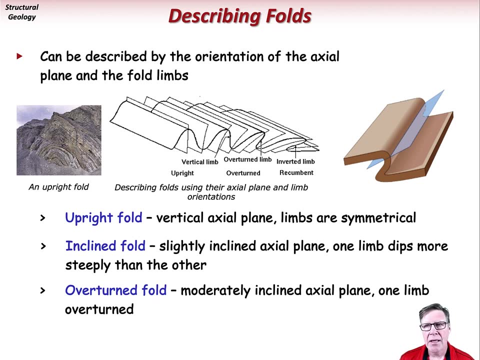 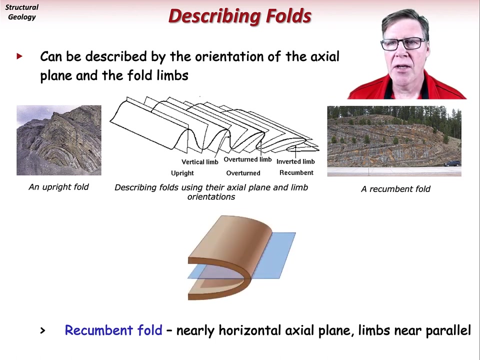 As the axial plane starts to tilt over, the forward limb, becomes steeper and steeper until it becomes vertical. An overturned fold is one where the axial plane exceeds a certain tilt angle, causing the forward limb to pass through vertical and become overturned. A recumbent fold is one where the axial plane is essentially horizontal or laying down. 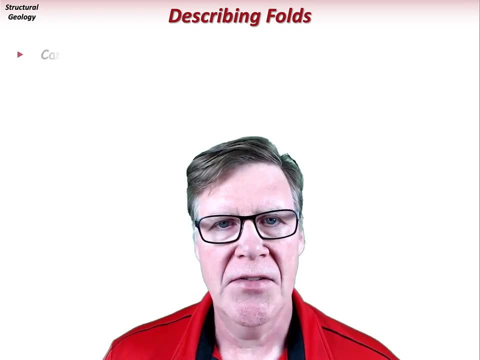 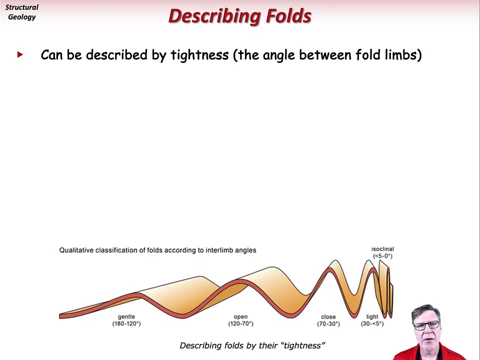 Another parameter that describes the shape of a fold is its tightness, controlled by the angle between the fold limbs. The differences in fold tightness are readily apparent in this figure of upright folds. Gentle folds are broad folds that have 180 to 120 degrees between fold limbs. 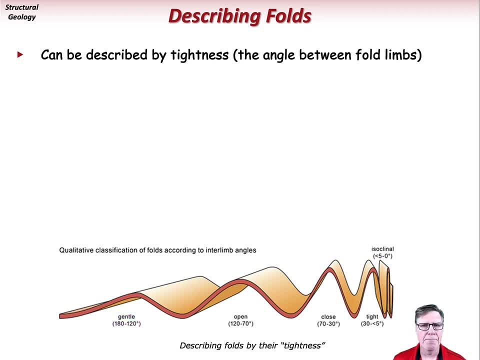 The limbs of these folds dip gently away from the axial plane. Open folds are common folds that have 120 to 120 degrees. Open folds are common folds that have 120 to 120 degrees. Open folds are common folds that have 120 to 120 degrees. 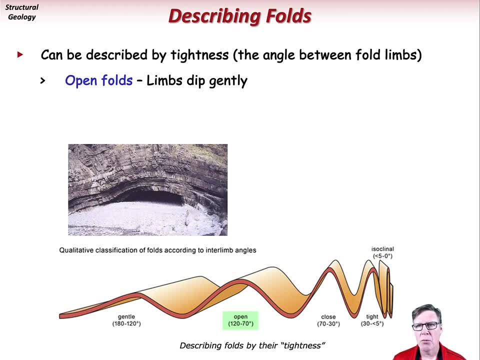 Open folds are common folds that have 120 to 170 degrees between the fold limbs, which dip more steeply away from the axial plane. Closed folds have 70 to 30 degrees between the fold limbs, which dip even more steeply away from the axial plane. 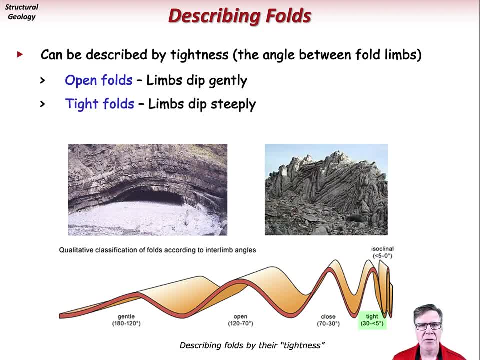 Tight folds have 30 to less than 5 degrees difference between fold limbs, which dip again even more steeply away from the axial plane. Closed folds have 30 to 30 degrees difference between fold limbs, which dip even more steeply away from the axial plane. 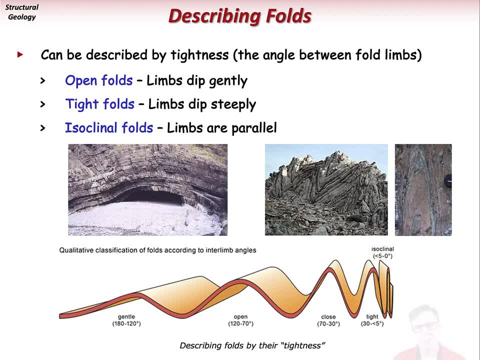 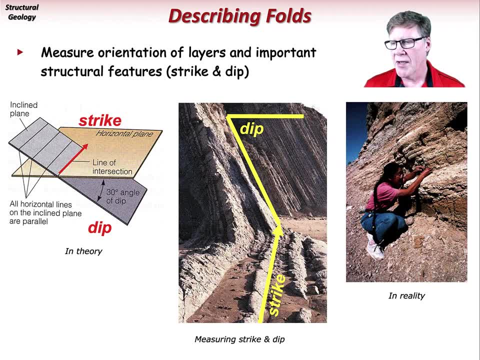 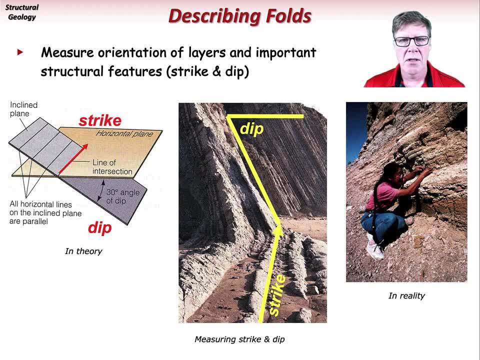 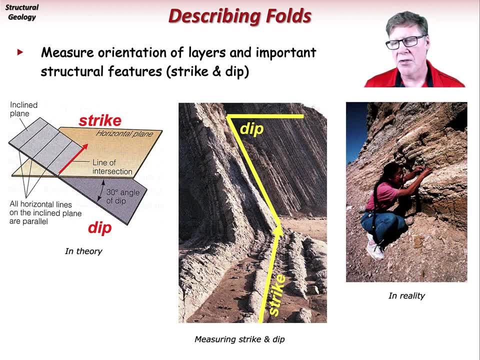 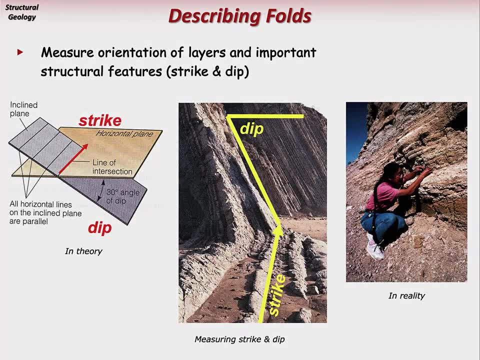 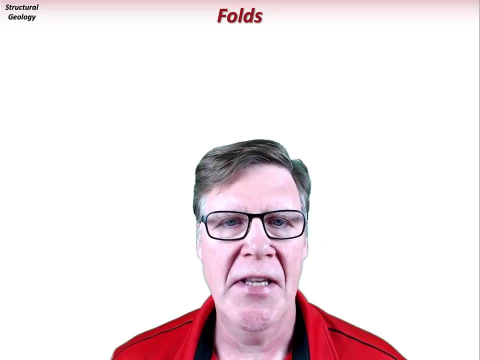 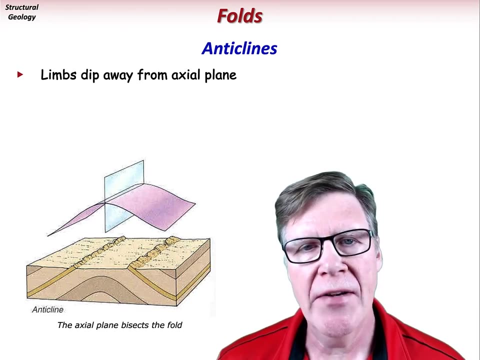 Closed folds have 30 to 30 degrees difference between fold limbs, which dip even more steeply away from the axial plane. One basic type of fold is the anticline, where the fold limbs dip away from the axial plane. Block diagrams like this are great for showing folds both in cross-sectional view from the 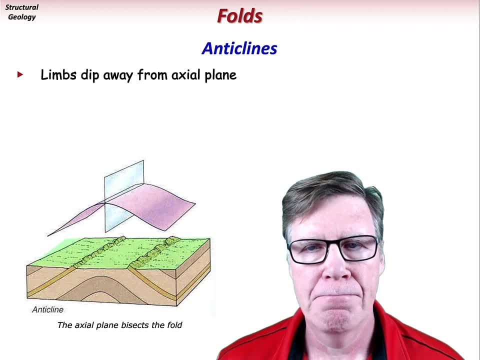 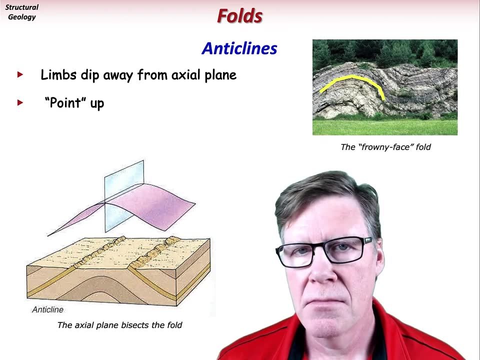 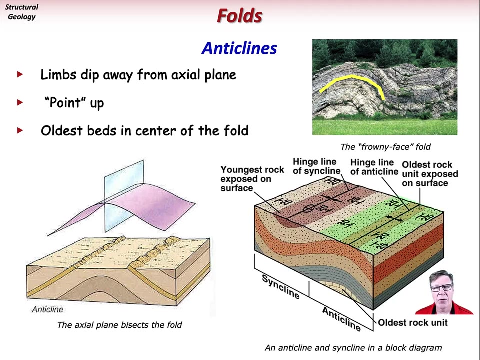 side and in map view from the top, In cross-section an anticline points up or forms a frowny face. In map view, the layers of an anticline dip away from the fold axis. An anticline map symbol may be drawn along the fold axis. 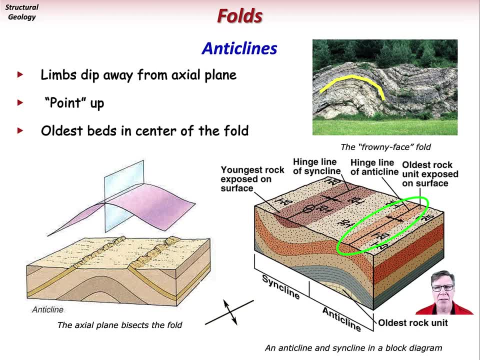 It has arrows pointing away from the fold axis in either direction to denote the dip direction of each fold limb. Also, in map view you can look at the ages of the different layers to tell what kind of fold you have. An anticline has the oldest layers exposed in the center of the fold along the fold axis. 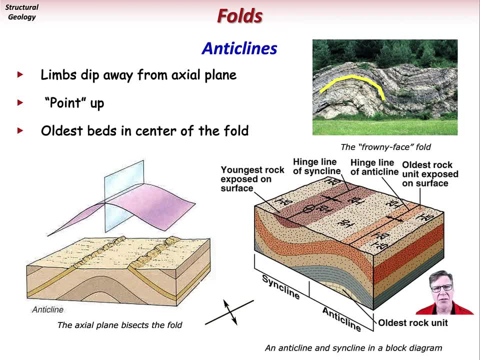 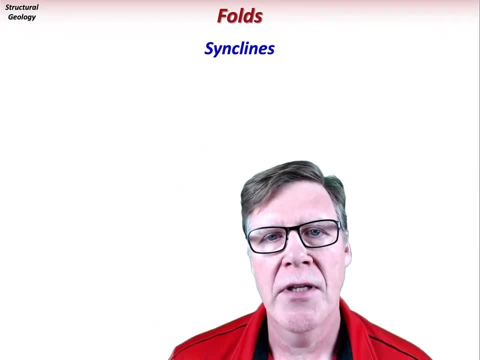 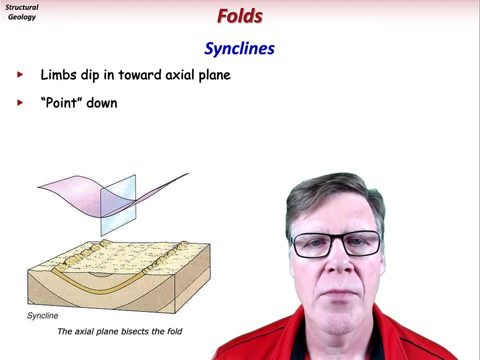 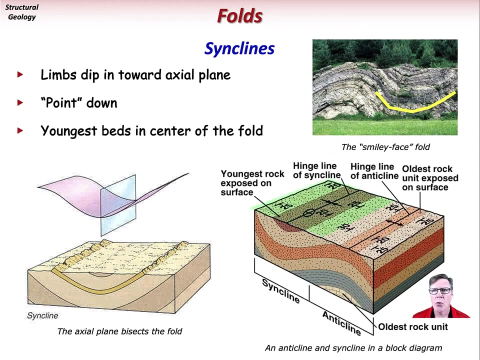 and the layers get progressively younger away from the fold axis. Another basic type of fold is the syncline, where the fold limbs dip toward the axial plane. In cross-section, a syncline points down or forms a smiley face In a map view of a syncline. the layers dip toward the fold axis on either side of the 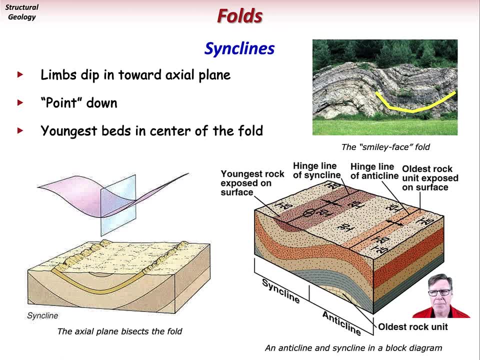 fold axis. A syncline map symbol may be drawn along the fold axis and it has arrows pointing up and down. This is a kind of syncline: has arrows pointing toward the fold axis to denote the dip direction of each fold limb. Also, in map view the youngest layers of a sincline are exposed in the center of the fold. 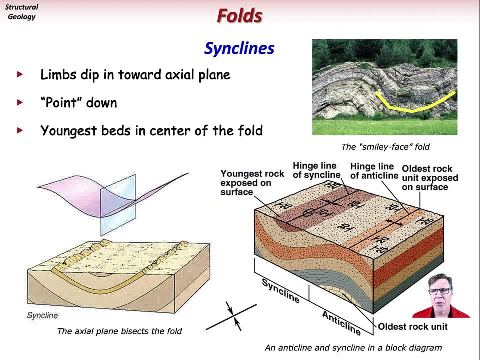 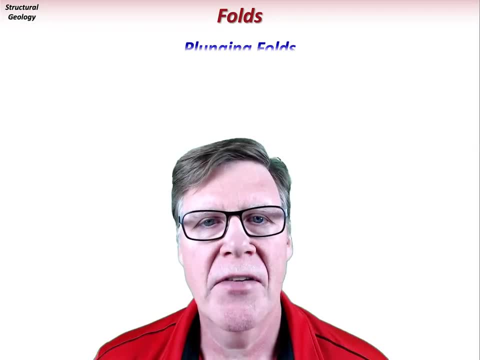 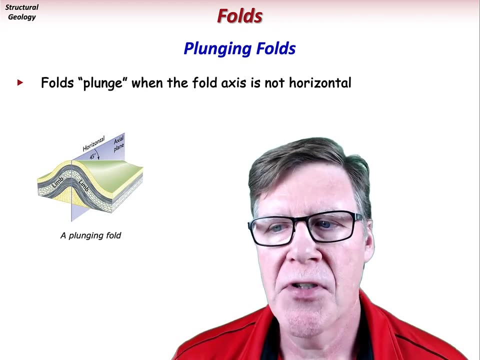 along the fold axis and the layers get progressively older in each direction away from the fold axis. A plunging fold is one that has a fold axis that is not horizontal but plunges downward. This produces outcrop patterns that are curved in map view. 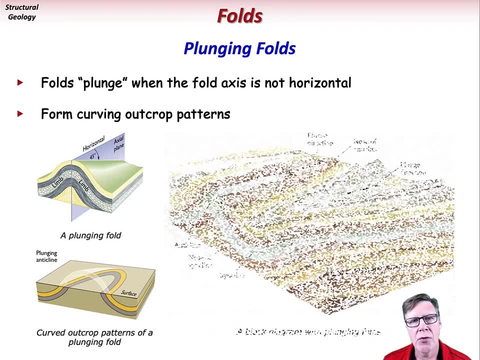 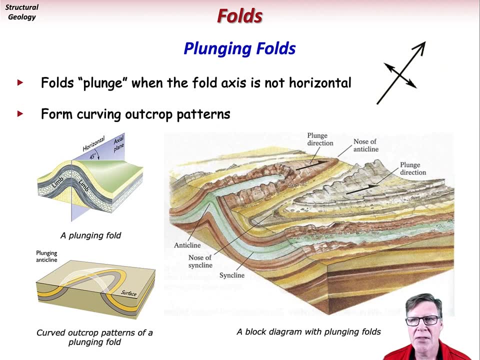 For plunging anticlines. the plunging fold patterns close or point in the direction of plunge. The map symbol for a plunging anticline is the same as an anticline map symbol with the added arrow pointing in the direction of plunge. 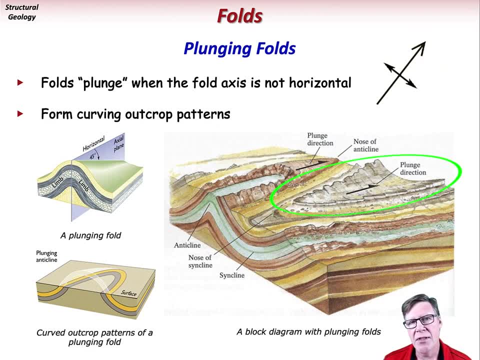 For plunging sinclines, the fold pattern opens in the direction of plunge and, conversely, points opposite the direction of plunge. The map symbol for a plunging sincline is the same as an anticline map symbol, with an added arrow pointing in the direction of plunge. 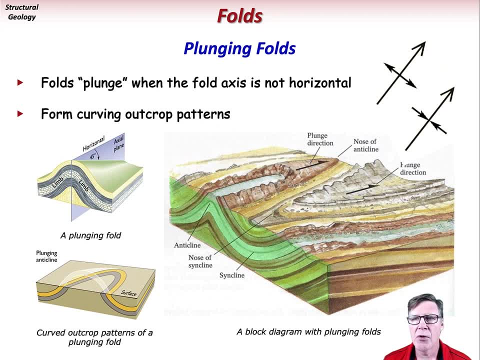 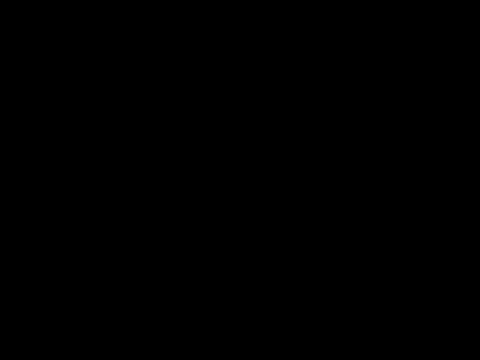 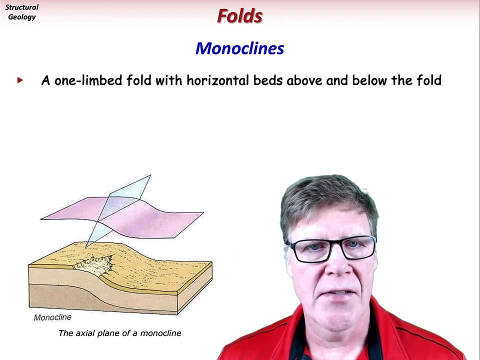 In cross-section plunging folds can look similar to non-plunging folds, but some views can actually show the plunging layers. Monoclines are one-limb folds that have horizontal beds above and below the fold axis. These folds are typically created by moving. 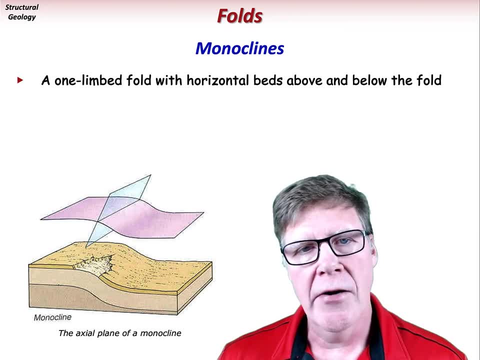 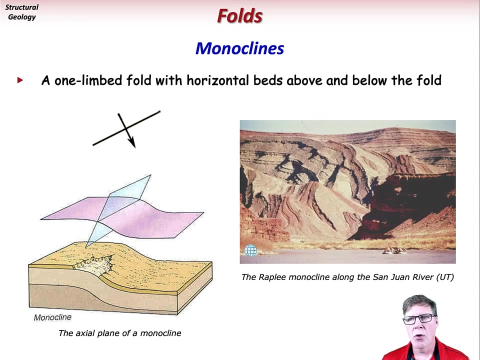 along underlying folds that deform the overlying layering. The map symbol for a monocline has a line following the fold axis, with the added arrow pointing in the direction of the downwarp. The Rappley monocline is a world-class monocline. 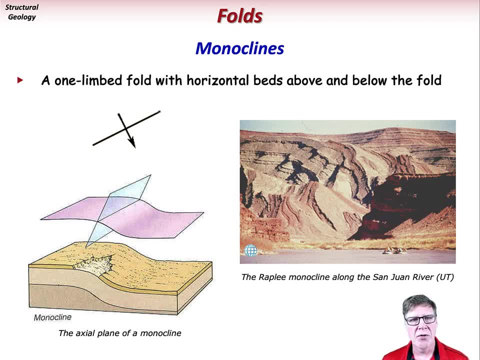 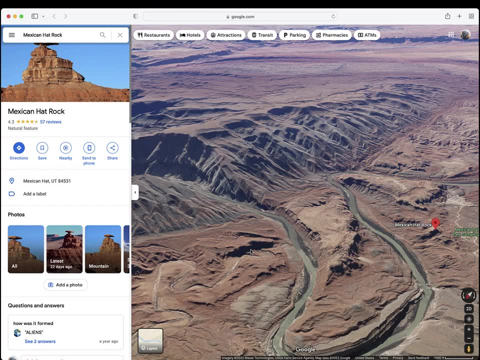 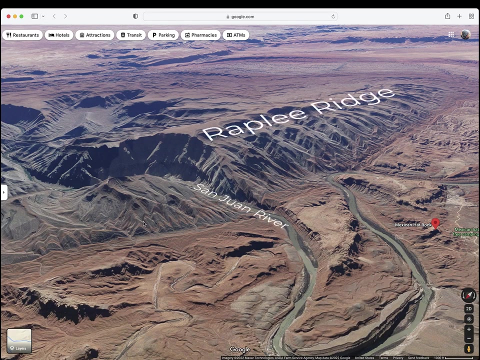 exposed along the San Juan River in southeasternmost Utah. Located along the San Juan River in southeastern Utah, Rappley Ridge displays world-class monoclinal folding along its western flank. The sedimentary rocks exposed here include the Pennsylvanian Hermosa group. 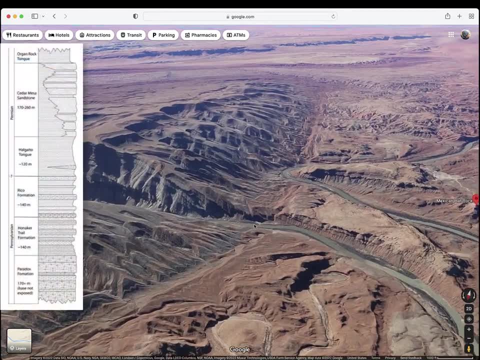 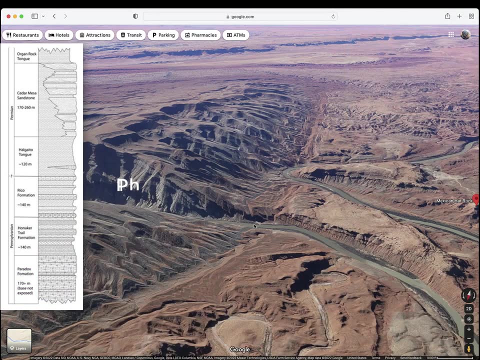 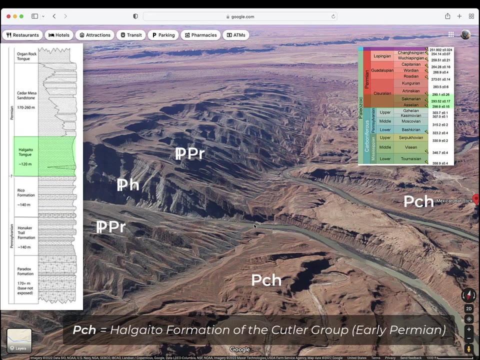 forming the deepest exposed rocks in the core of the monocline. These are overlain by various areas of the monocline. These are overlaid by various areas of the monocline by various members of the Rico Formation and the Al Gaito Formation, Redbeds and the Cedar Mesa. 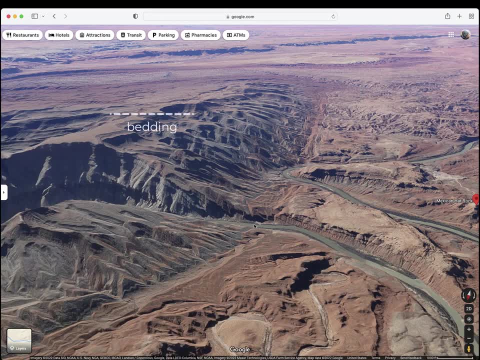 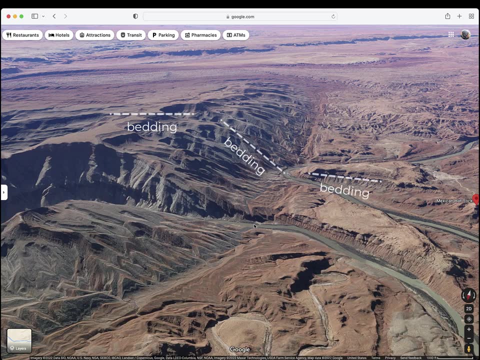 Sandstone. These layers are horizontal along the ridge crest and then dip as much as 40 degrees through the fold until dips flatten again at the bottom, with the Mexican Hat Sincline located to the west. This fold formed as a result of the compressional tectonics of the latest Cretaceous. 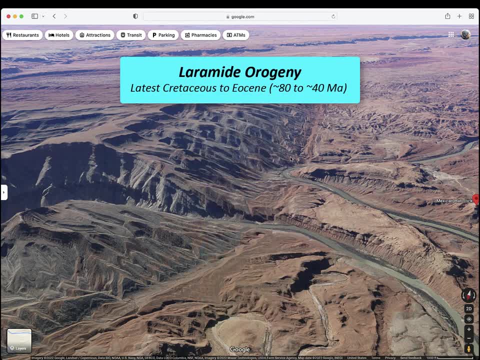 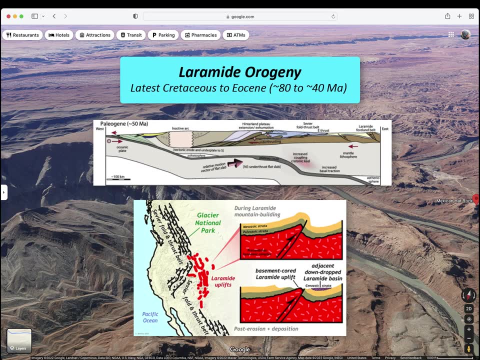 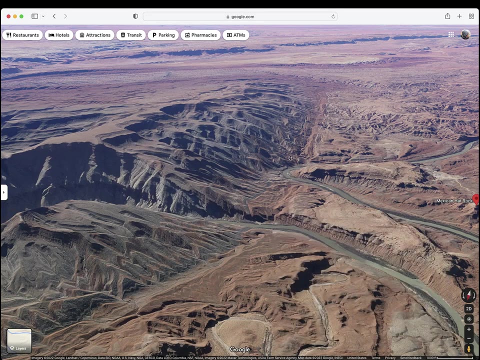 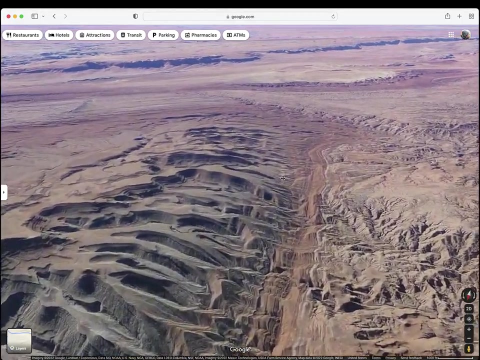 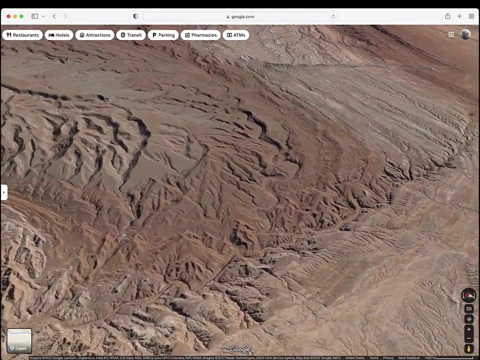 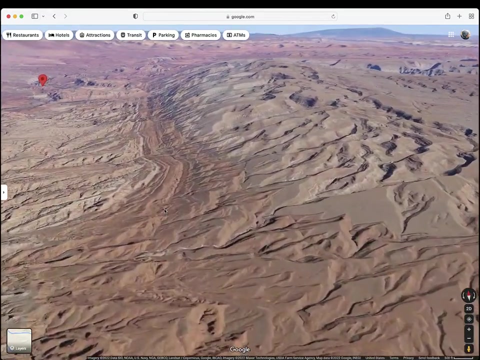 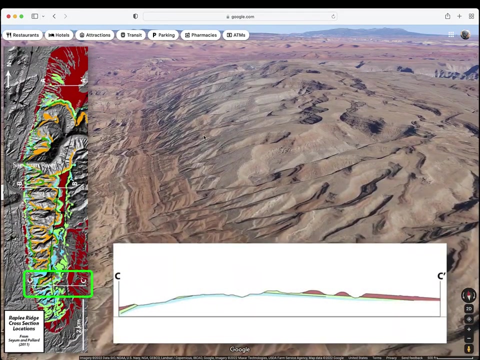 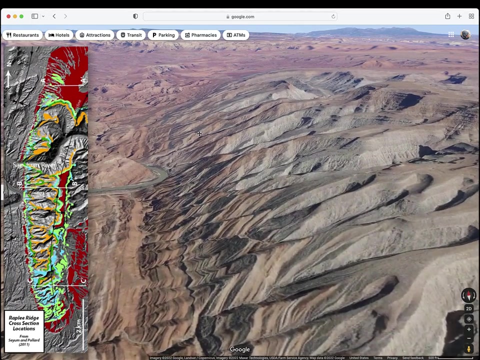 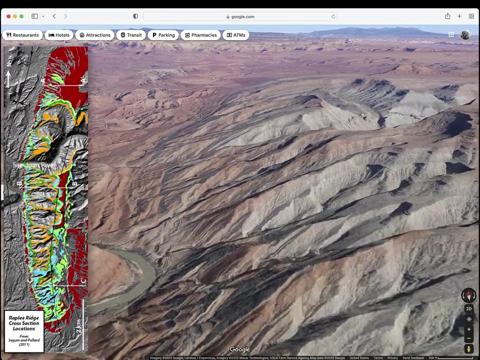 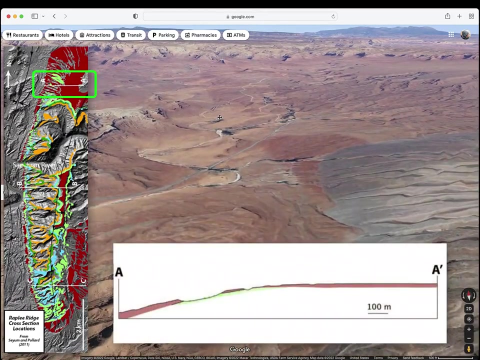 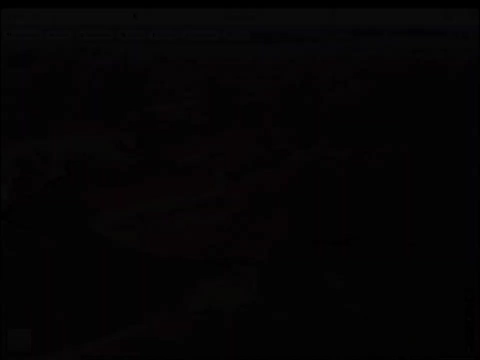 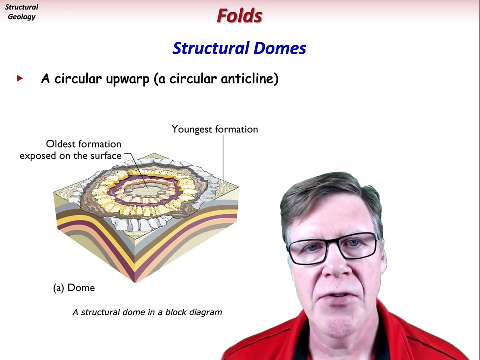 to Eocene Laramide Orogeny, where movement along deep-seated reverse faults caused monoclinal folding of the overlying Paleozoic and Mesozoic sedimentary rocks. For more information, visit wwwFEMAgov. Major Moscow Structural domes are large circular upwarps that are essentially equivalent to circular. 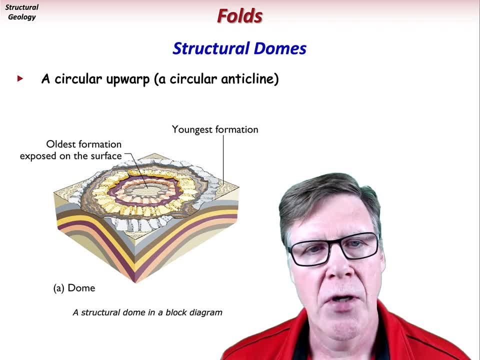 anaclines. Like anaclines, structural domes point upward in cross-section. In map view, the oldest layers are located in the center and dip away from the center in all directions. The map symbol for a structural dome has four arrows pointing outward away from the center of the fold. 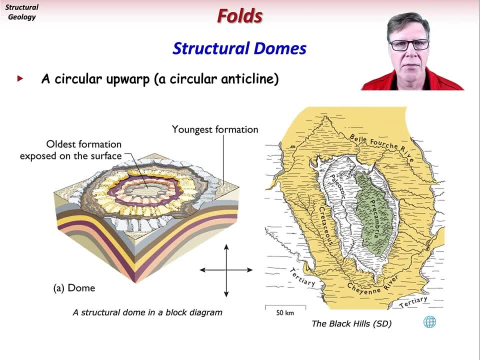 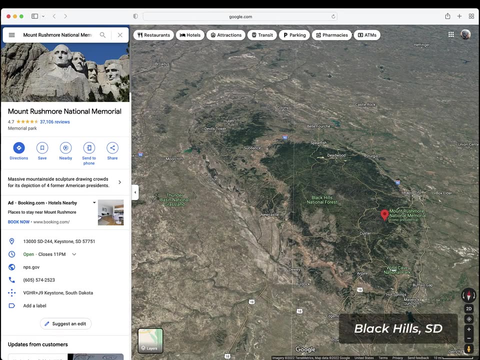 The Black Hills of South Dakota are located in the center of a structural dome. Indeed, Mt Rushmore is carved into the Precambrian rocks exposed at the core of this structure. Here are the Black Hills of western South Dakota and eastern Wyoming. 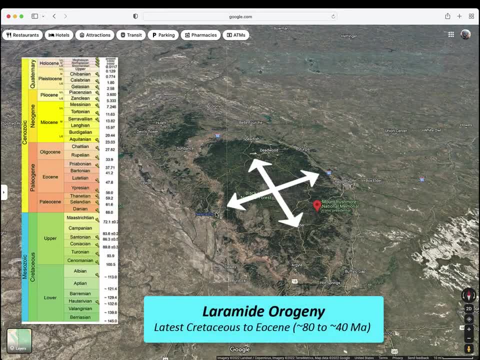 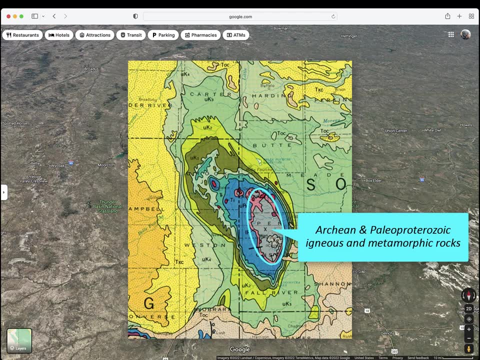 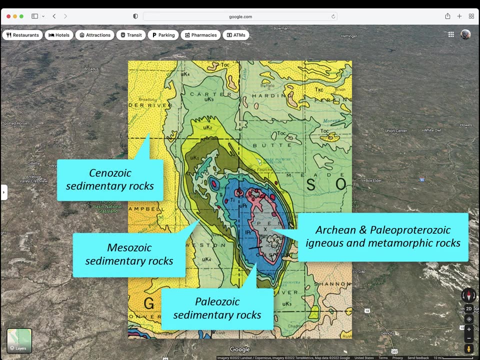 This structural dome was formed during the latest Cretaceous to Eocene Laramide Orogeny and is cored by Archean and Paleoprotozoic igneous and metamorphic rocks covered and surrounded by progressively younger Paleozoic, Mesozoic and Cenozoic sedimentary rocks. 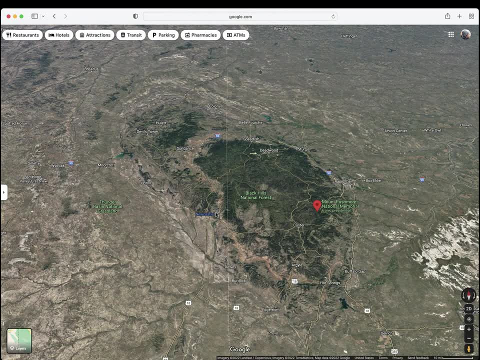 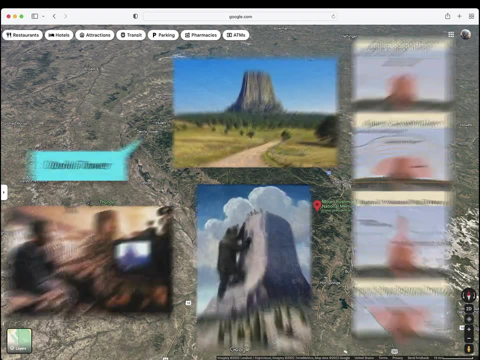 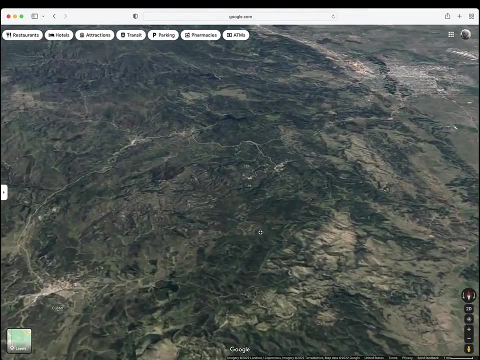 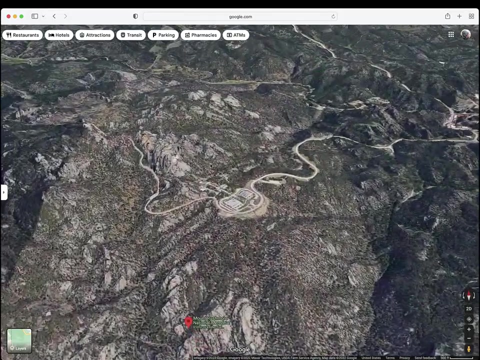 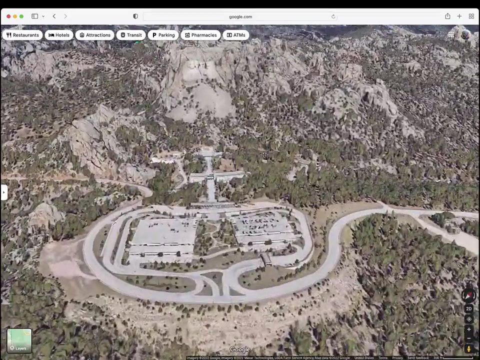 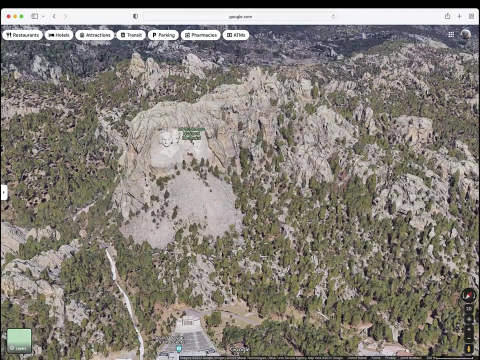 Laramide Eocene intrusions are also present, including at Devil's Tower. The Black Hills are a signpost for the 73th anniversary of the Great Depression and are part of the history of the Great Depression. The Black Hills are also a symbol for the 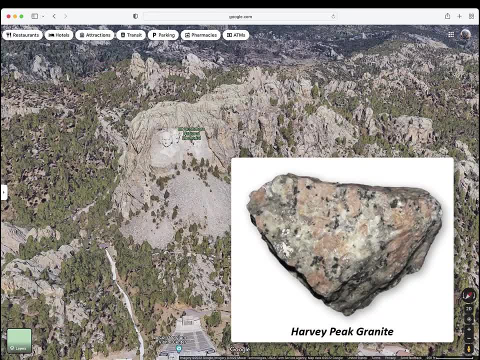 history of the Great Depression. Mount Rushmore is carved into the Harvey Peak granite, which has an age of 1,700 million years. Mount Rushmore is carved into the Harvey Peak granite, which has an age of 1,700 million years. 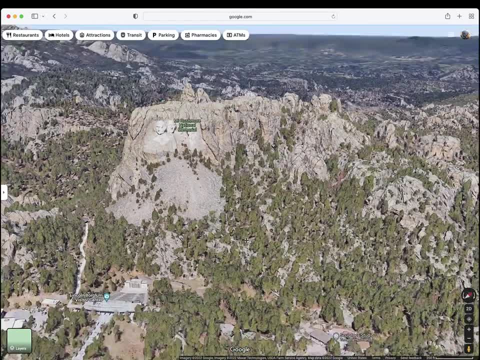 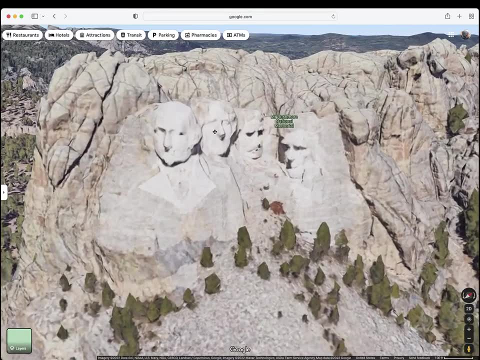 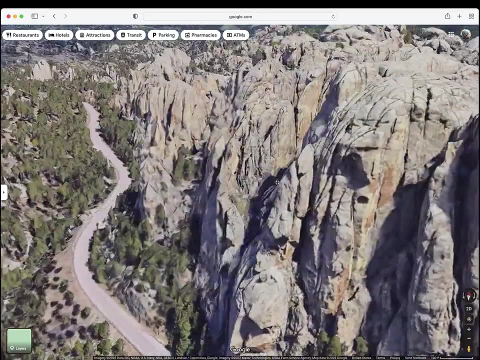 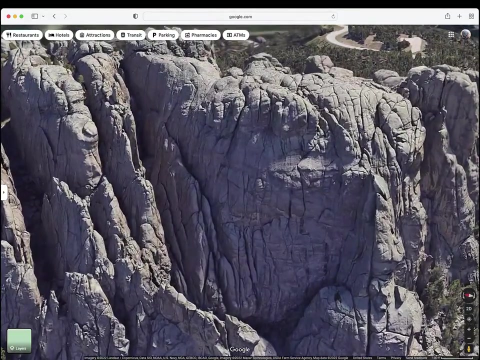 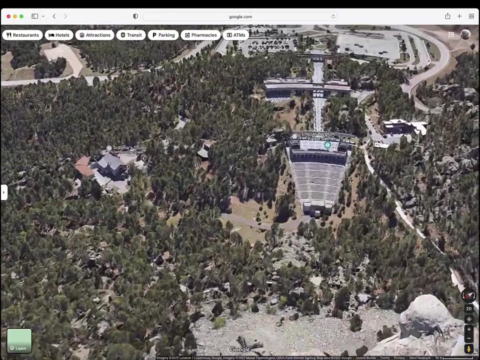 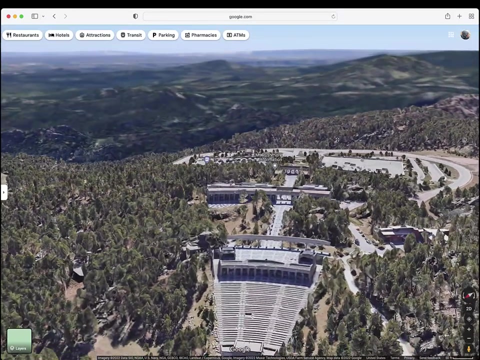 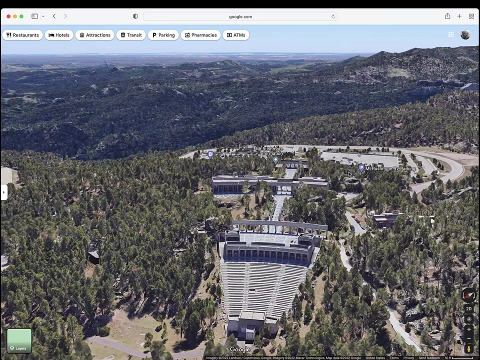 This coarse-grained Muscovite barren granite is host to the 60-foot-high presidential sculptures carved between 1927 and 1941.. If you ever wondered, this is the view the fellas have to the east, toward the Great Plains. 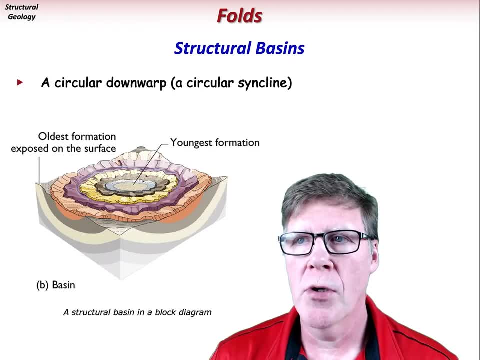 Structural basins are large circular downwarps that are essentially equivalent to circular synclines. Like synclines, structural basins point downward in cross-section. In a map view, the youngest layers are located in the center and dip toward the center from.